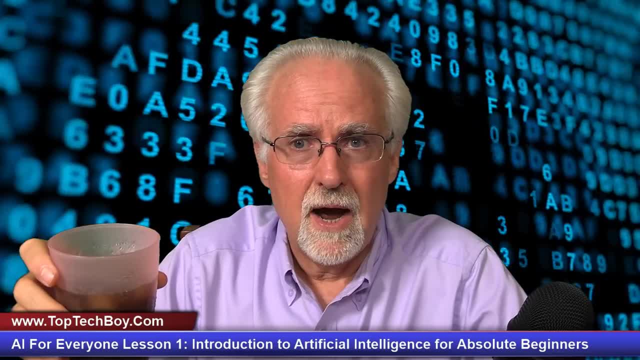 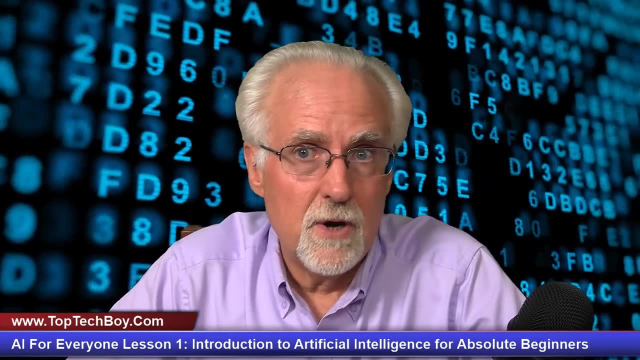 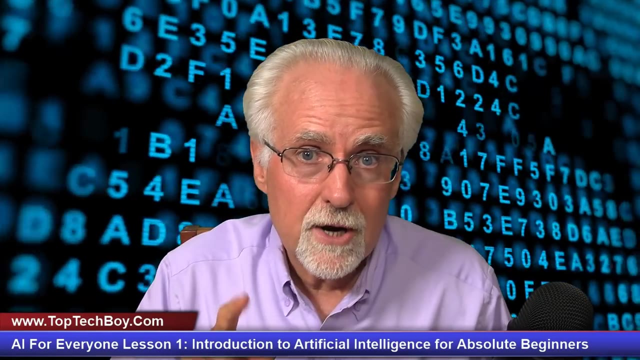 That is straight up: black coffee poured over ice, no sugar, no sweetener, none needed. Now, as you're getting out your coffee, as always, I want to give a shout out to you guys that are helping me out over at Patreon. It is your support and your encouragement that keeps this great. 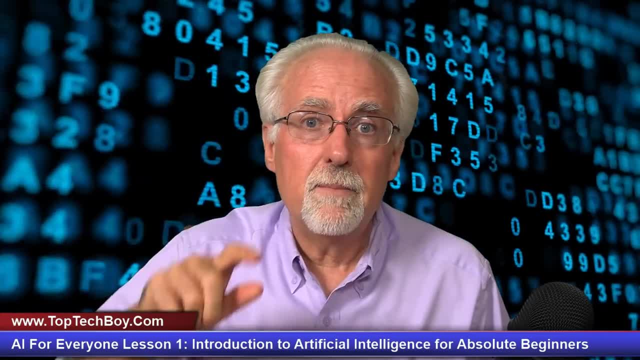 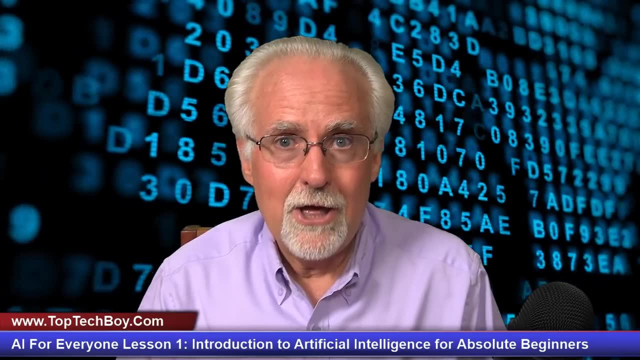 content coming. You guys that are not helping out yet think about looking in the description down below. There is a link over to my Patreon account. Think about hopping on over there and hooking a brother up. But enough of this shameless self-promotion, Let's jump in and let's talk. 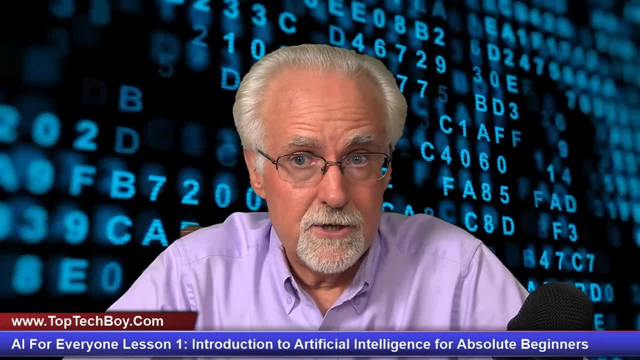 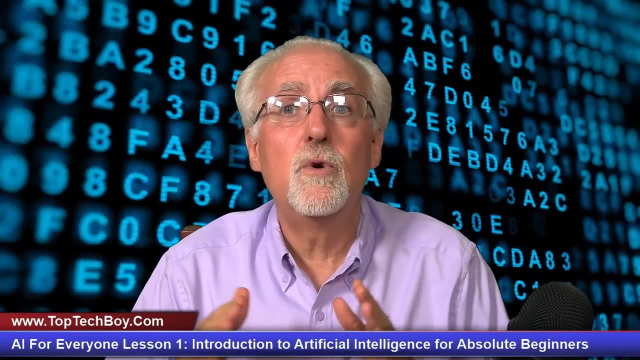 about what we are going to learn. I'm going to teach you artificial intelligence. This is going to be an entire class. It is going to be a series of lessons And in today's lessons, I'm going to give you an introduction to the. 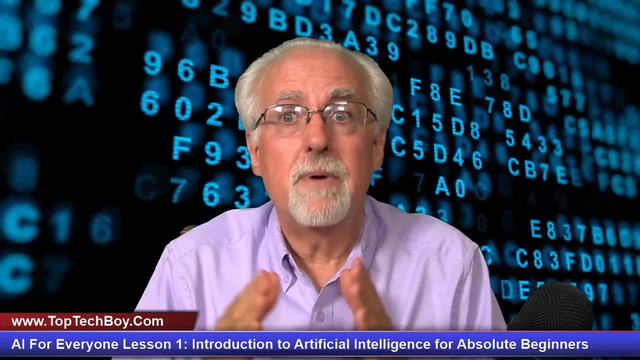 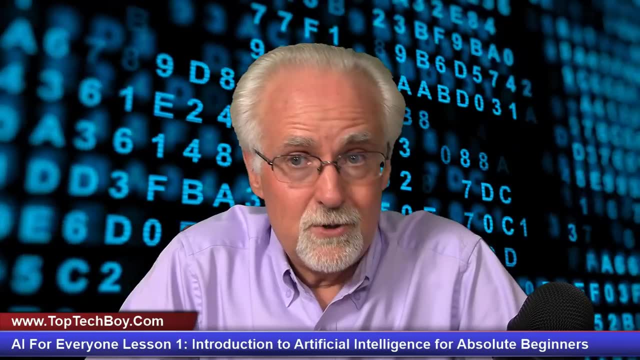 overall class. So we're not going to be actually coding today, but I'm going to be telling you what you will learn if you take this class. So, first of all, if I'm going to teach you about artificial intelligence, what is artificial intelligence? Now I could give you the computer. 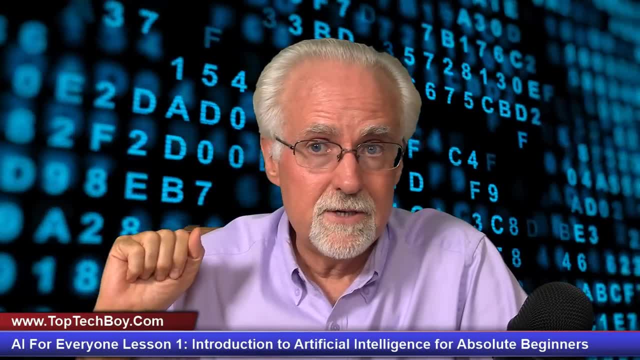 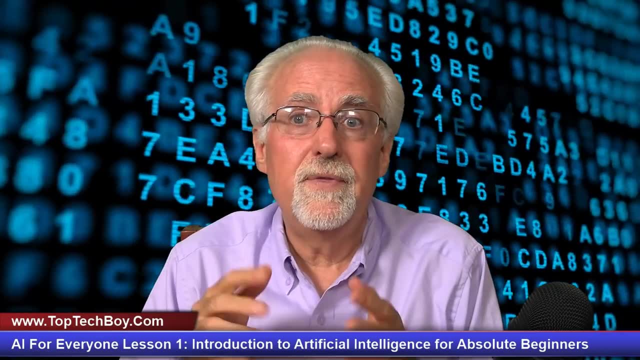 science definition or the MIT PhD type of thing. but I'm going to give you the artificial intelligence definition, But instead I'm just going to give you kind of a common sense definition. And the common sense definition to me is when the computer starts doing things that you would normally. 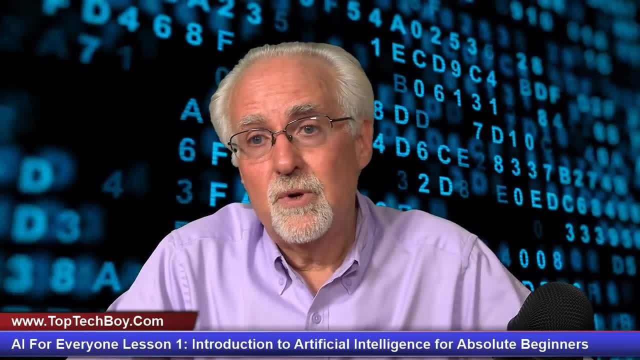 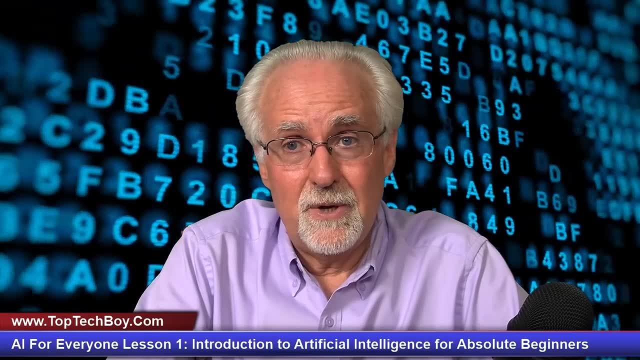 associate with a person doing So traditionally. if you had something like a picture, and the picture had cats and dogs in it, you could hand that picture to a three-year-old and the three-year-old could draw a circle around the cats- A two-year-old, a three-year-old could draw a circle around the. 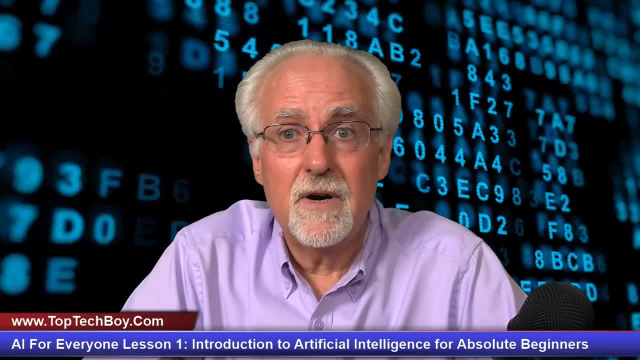 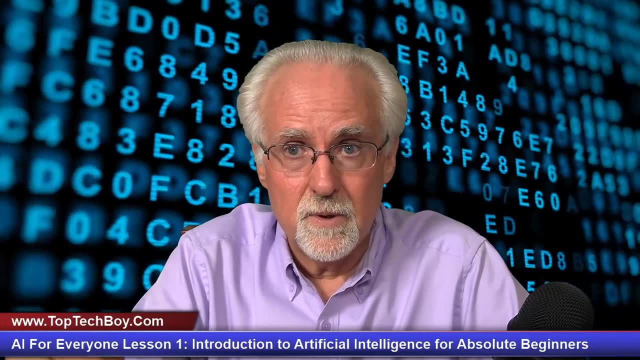 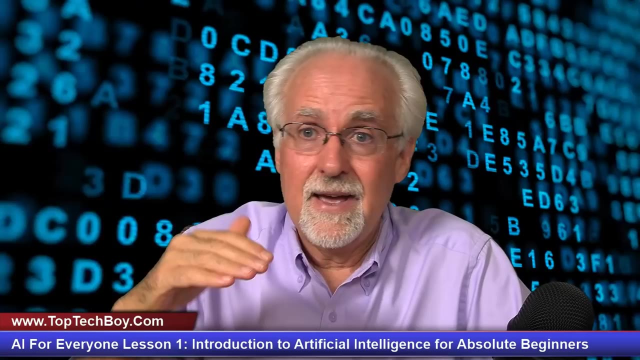 cats. That is something that is very easy to do, So I'm going to give you a common sense definition. But that is not something that comes easy or natural to a computer. Typically, a computer executes a very logical set of instructions and like: x equal three, y equal two, z equal x plus y. 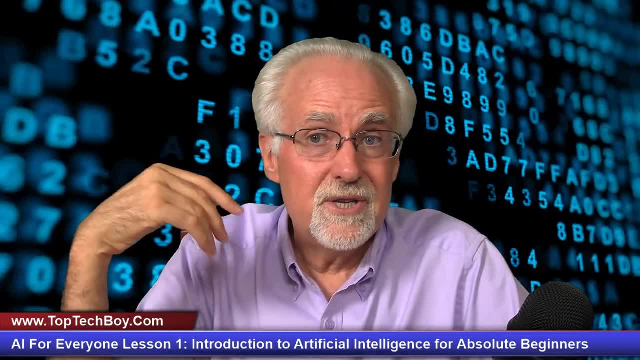 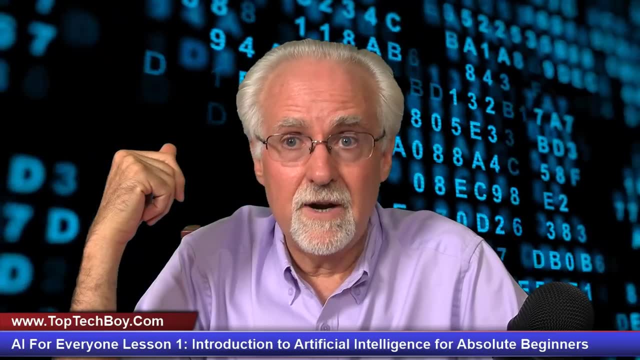 and then print z A very logical set of instructions, and the computer can work it perfectly, and the computer can work it quickly. but the computer can't think on its own very well, and so it is not going to know the difference between cats and 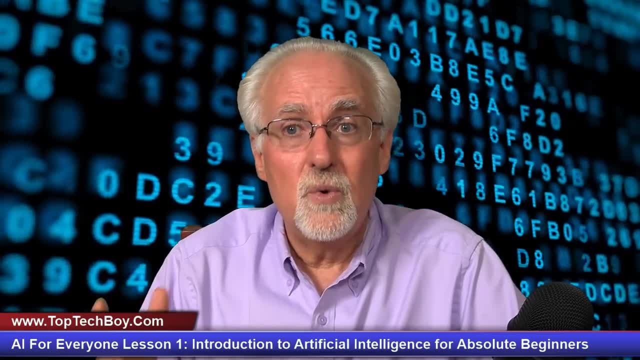 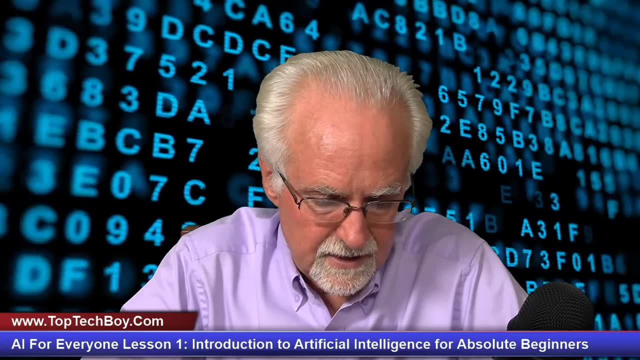 dogs. And so, as we can get a computer to start doing something like look at a picture and know the difference between the cat and the dogs, that is what we call artificial intelligence. Okay, let me give you another example. Let's say that if I get on the computer and I open, 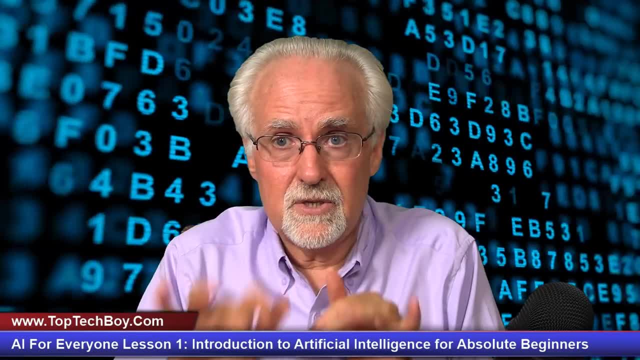 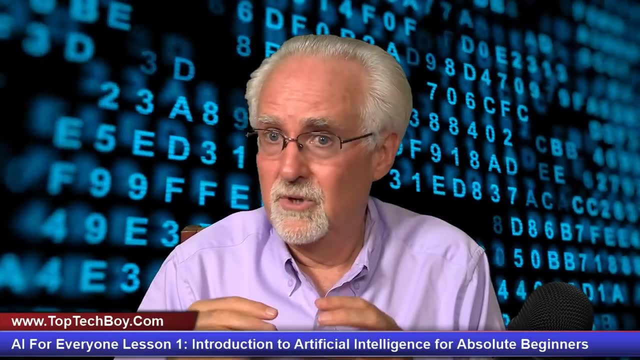 up Microsoft Word and I start typing and it takes those keystrokes and turns them into letters and words and paragraphs. that's what you would expect a computer to do. Does it really well? but it doesn't have to really think, It doesn't have to figure things out. 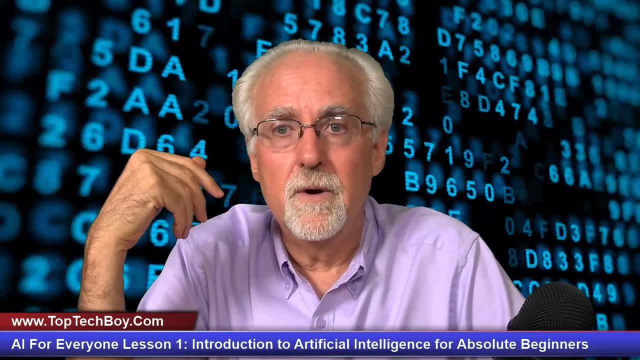 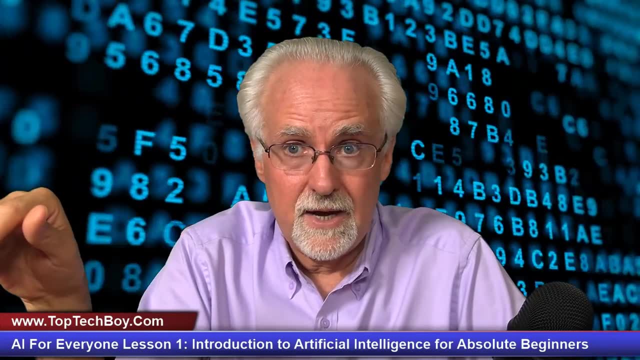 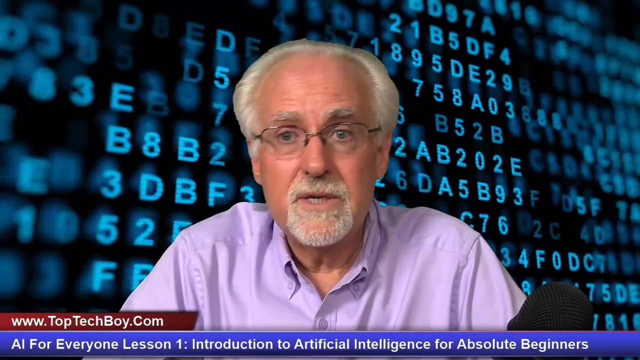 Now, on the other hand, if I speak into the microphone and the computer hears the sounds and then turns them into words, turns them into text, all of a sudden that starts being a little bit more like artificial intelligence. Or if we go one step further and it's not only turning 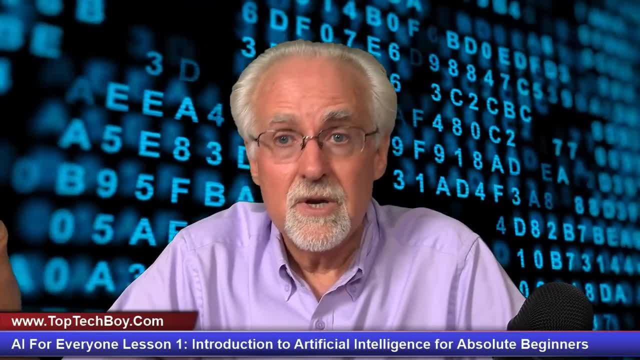 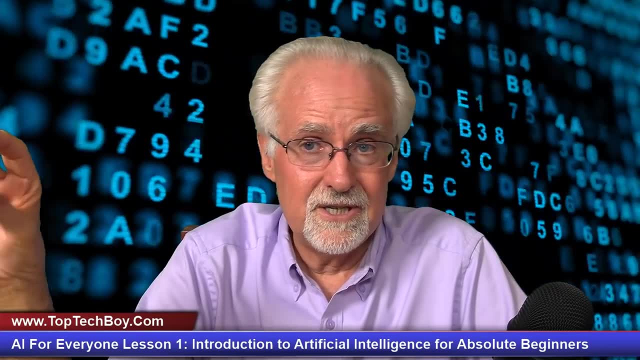 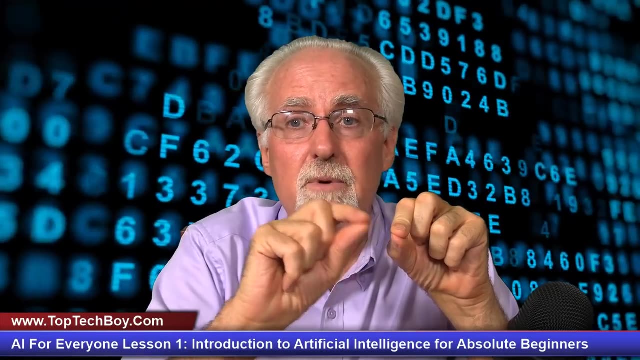 those sounds into a string of letters, but it's starting to discern what it is that you're saying. then that really starts being artificial intelligence. And so if I say what is the temperature in Albuquerque, And it turns that into text: W-H-A-T space, I-S space. 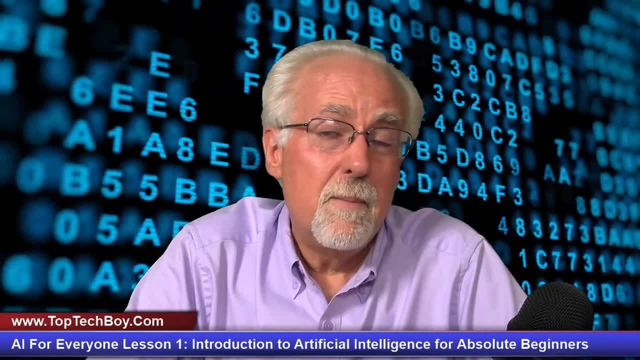 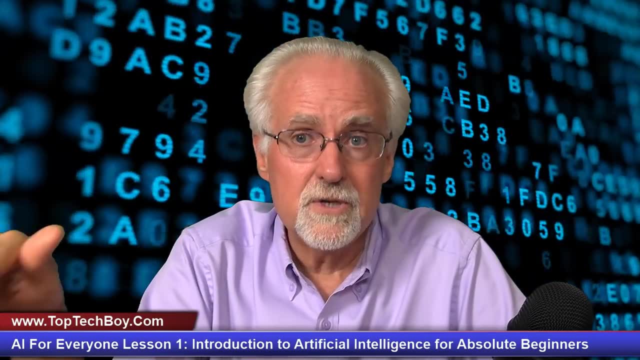 turns it into text. that's kind of showing a little bit of intelligence. But if I say what is the temperature in Albuquerque, And it not only turns that into a string of letters or a string of words but then perceives that you're asking it a question, 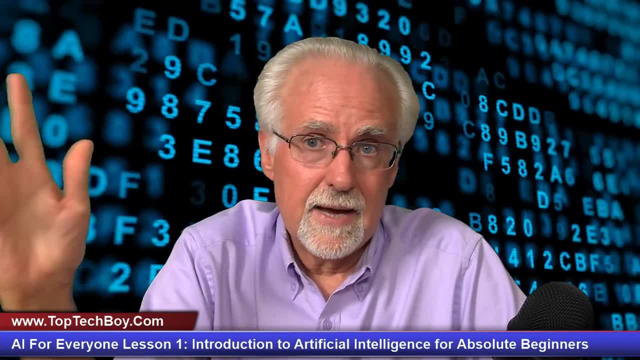 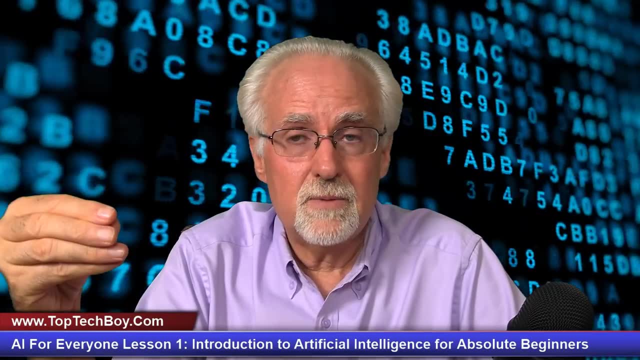 and then it goes out and it figures out where to look it up And it comes back and says the temperature in Albuquerque, New Mexico, this morning is 78 degrees. Now that starts being artificial intelligence. So that is what I consider artificial intelligence. 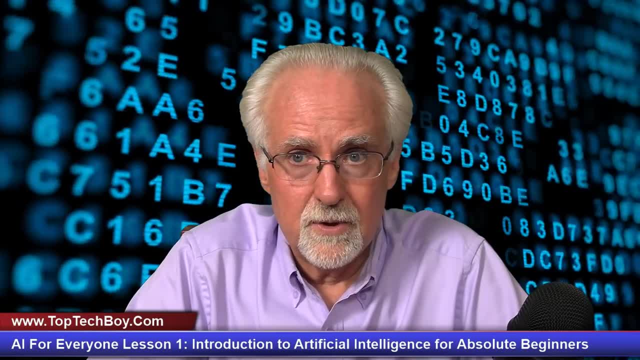 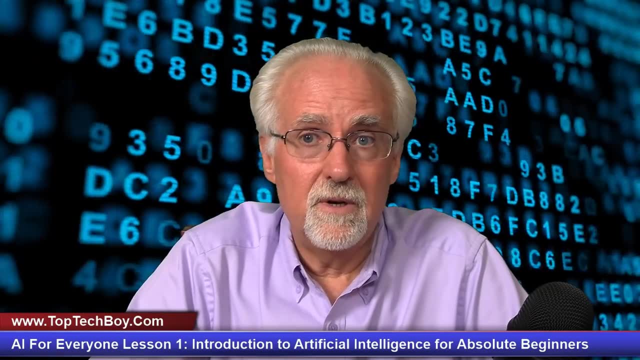 When the computer starts doing things that you would normally associate with a person, when it starts doing things that are very natural for a person to do and very unnatural for a computer to do. that's when I say the computer is starting to demonstrate. 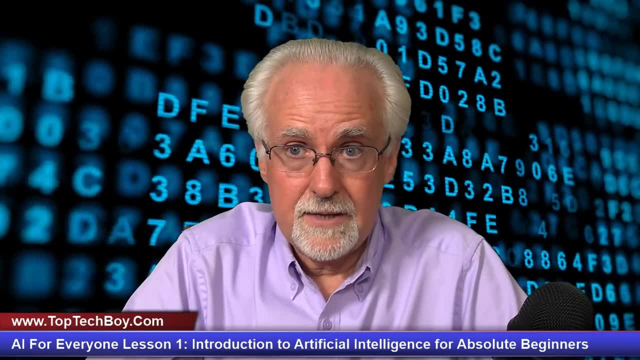 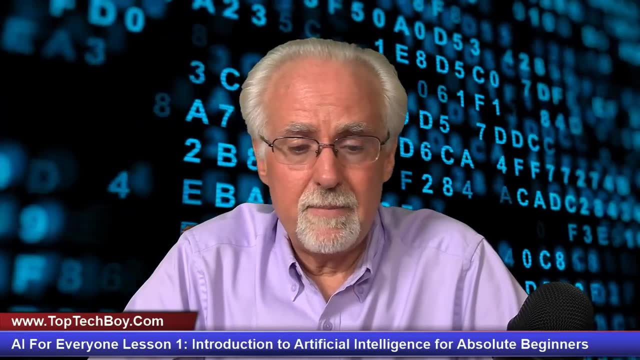 artificial intelligence. Okay Now, if you're going to take this class, what are the prerequisites? Okay, The prerequisites really are: you don't have to be an expert in programming, You don't have to be an expert in computers, but you do need to sort of have a little programming experience. 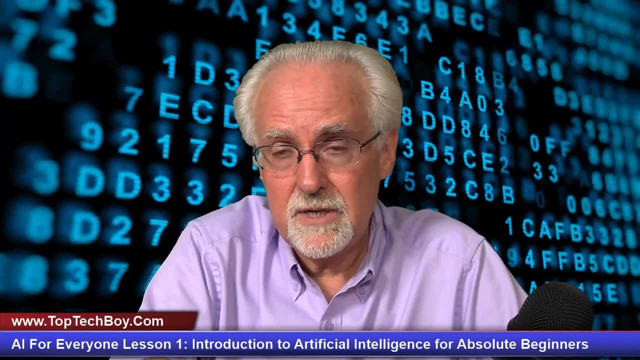 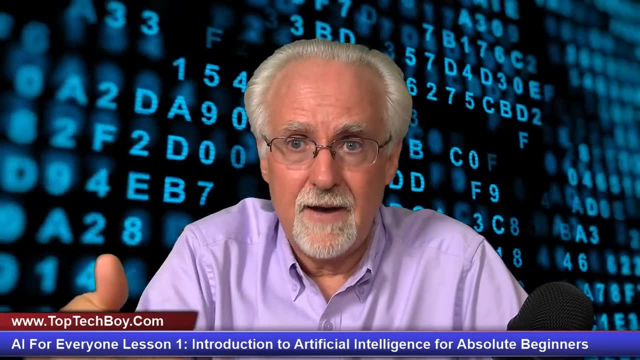 For example, if you followed along with me through the podcast, I'm going to show you a little bit of Python series of lessons. You're good to go, man. You're really ready. You're right on track to do this, and to find this series of lessons in class is very easy If you've taken my Arduino. 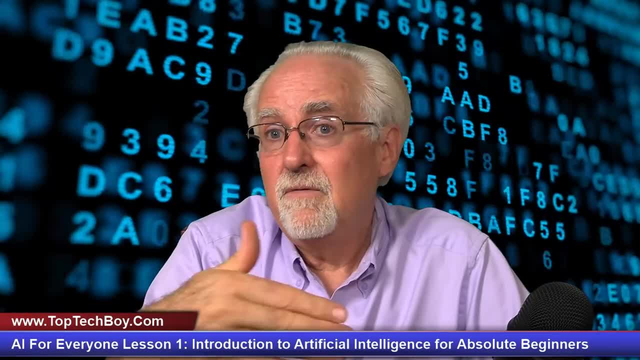 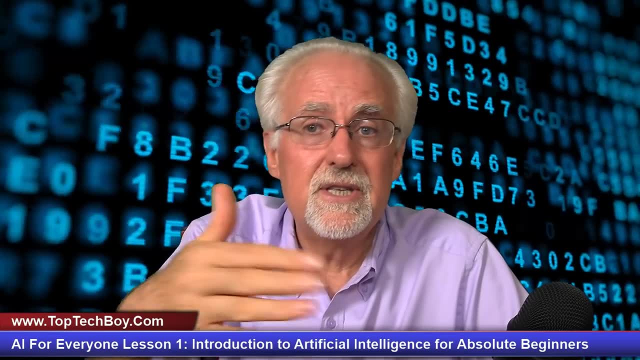 lessons. you're going to be pretty much ready to go in this class. If you've taken the Arduino, it might be helpful if you had a little familiarity with Python. Maybe you took a few of the Python lessons. Then, as I'm jumping in and doing things in Python, you're going to be. 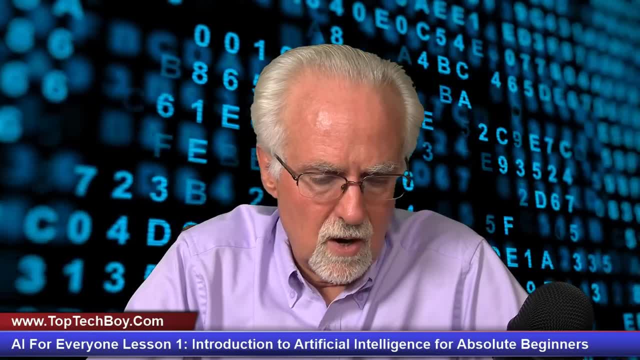 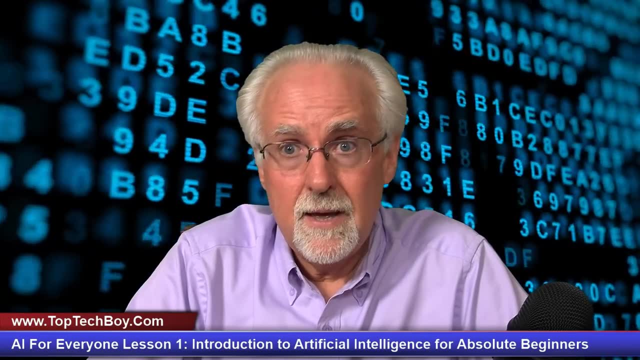 ready for it. So if you're going to be doing things in Python, you're going to be ready for it. But don't really assume- I'm not assuming- that you are a computer expert. So what do I assume as I am making these lessons for this class? I'm assuming that you're a hard worker. I'm 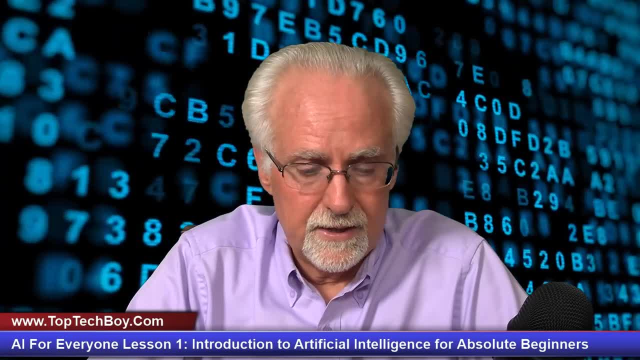 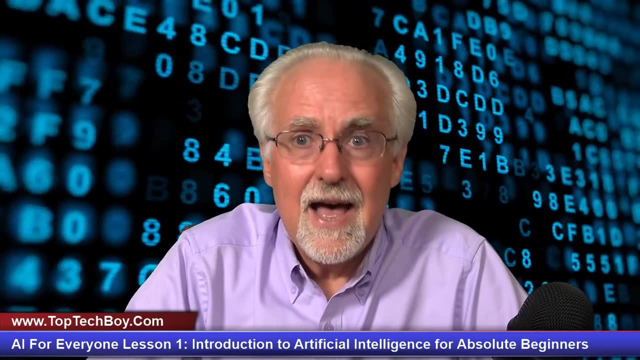 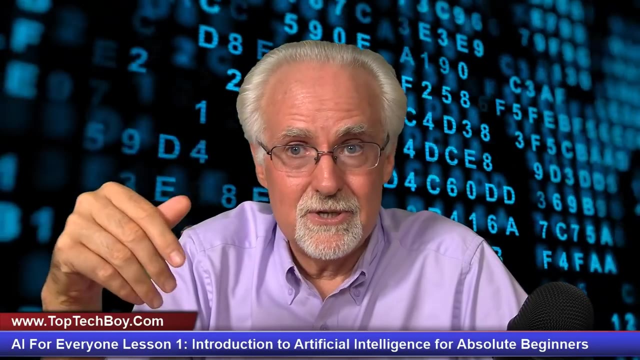 assuming that you're willing to try. I'm assuming that you are willing to listen. I do not assume that you already have your PhD from MIT in computer science. I do not assume that you know the hundred magic words of artificial intelligence, right? I'm assuming that. 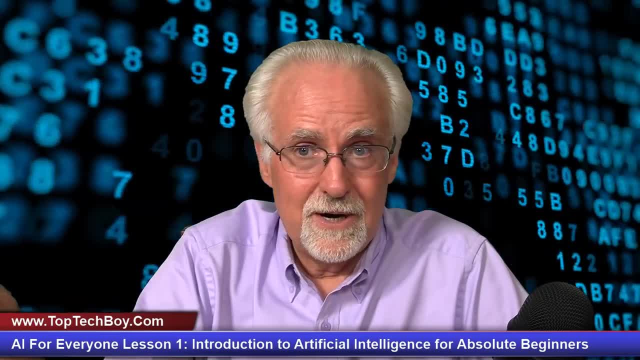 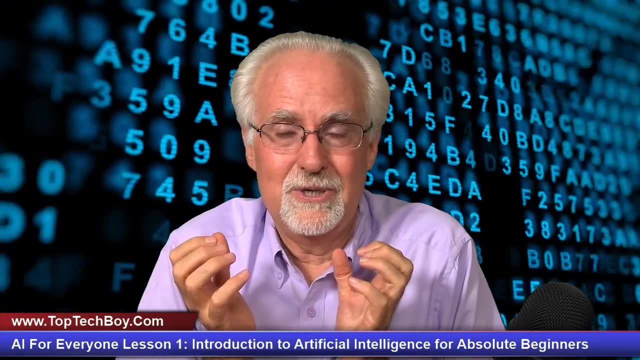 you're a smart guy willing to learn, but that you don't already know all that stuff. And man, I wanted to learn artificial intelligence and I can't tell you how hard it was. It is like a secret priesthood and this priesthood has a hundred words And anytime they define. 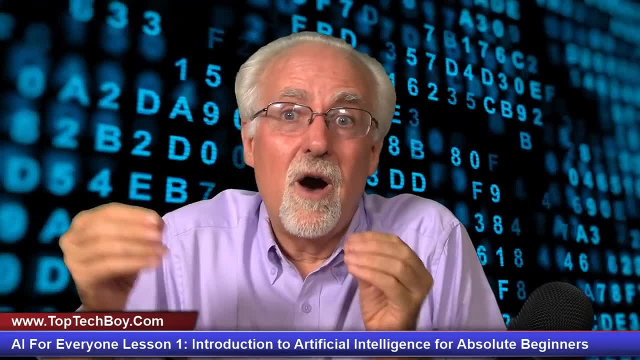 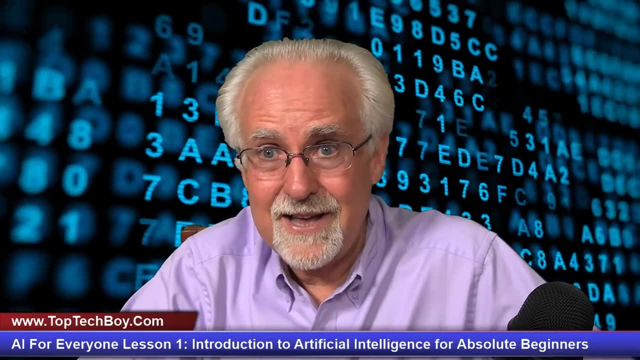 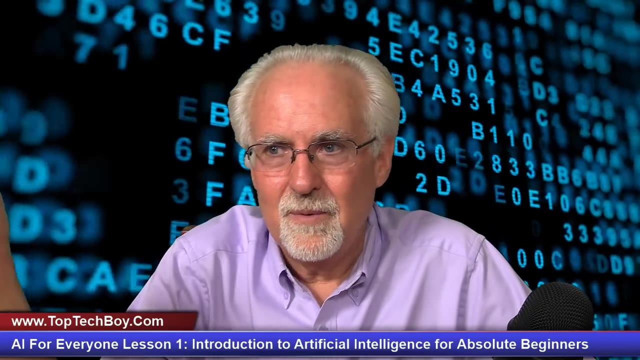 one of those hundred magic artificial intelligence words. they always use one of the other hundred words to define it, And so you're just going in circles with all these things that you don't understand about TensorFlow and cafe models and and deep neural networks and deep learning and machine learning and all these different things. 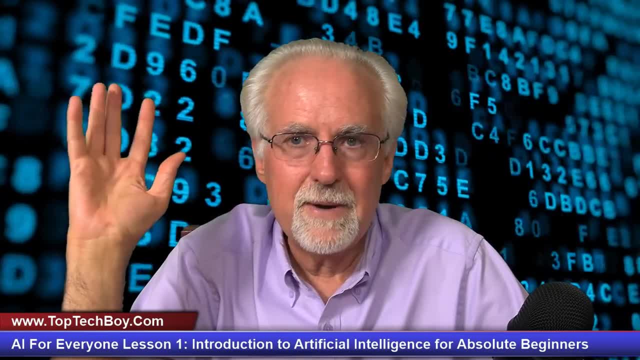 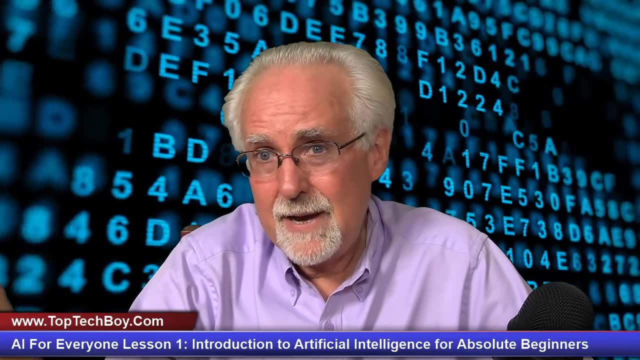 And they always define those things in terms of other things that you've never heard about. So it's really hard to find like: okay, I'm a programmer, I know a little bit about computers, I know a little bit about Python and Arduino. How do I break into this field of artificial? 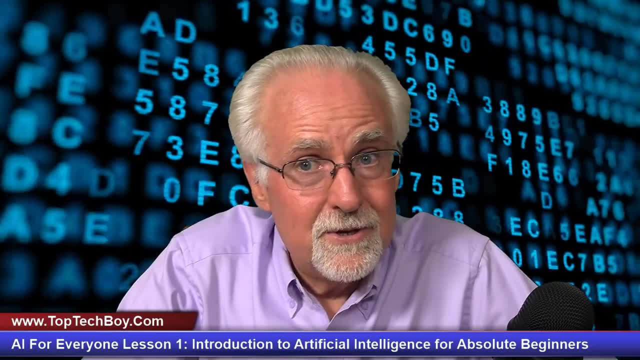 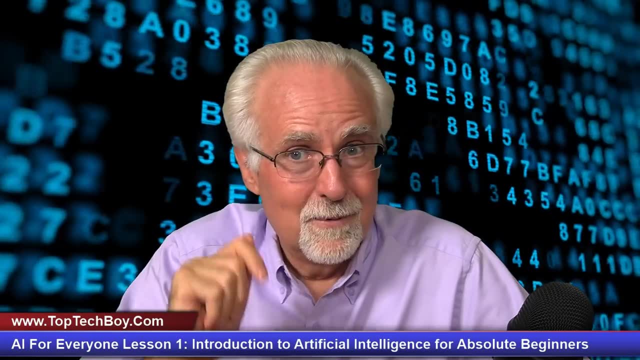 intelligence. That's what this class is going to do. There's a lot of people that know a lot more than I do about artificial intelligence, but I know how to teach and the things that I know. I can show you how to do, and we're going to have some fun along the way. Okay, I promise I'm not. 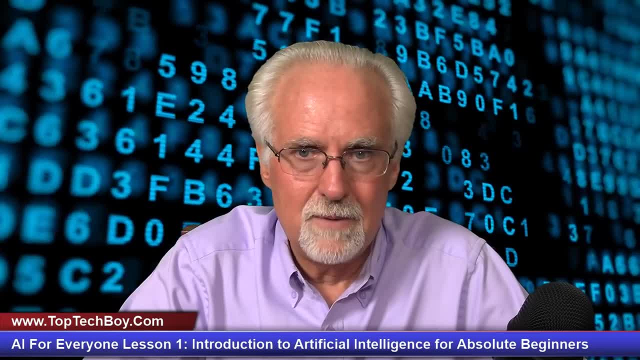 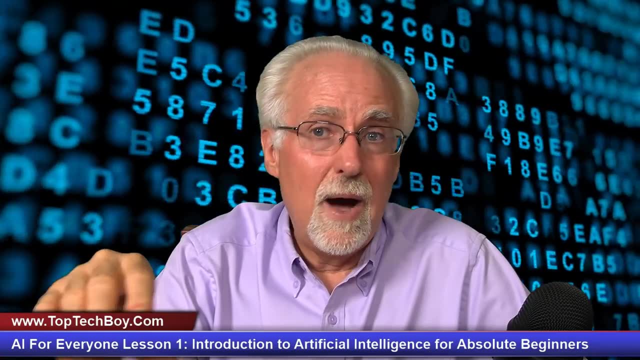 going to leave anyone behind. I promise that I am not going to leave anyone behind. Okay, this class is going to be based on a Windows PC. I'm going to be running Windows 10.. And why do I do that? Because I've done some artificial intelligence lessons in the past on 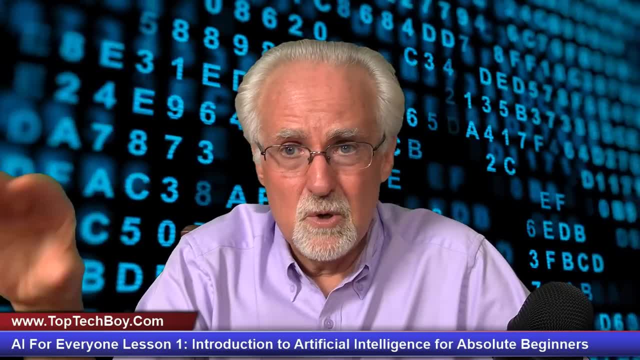 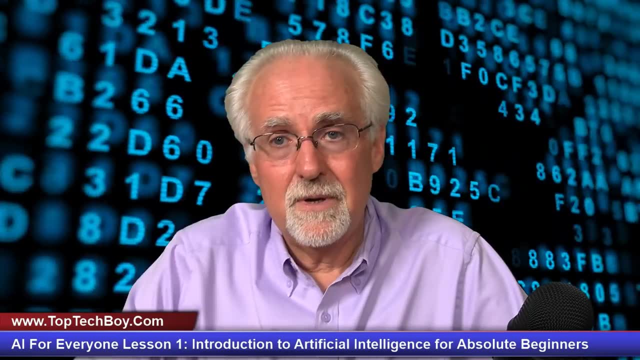 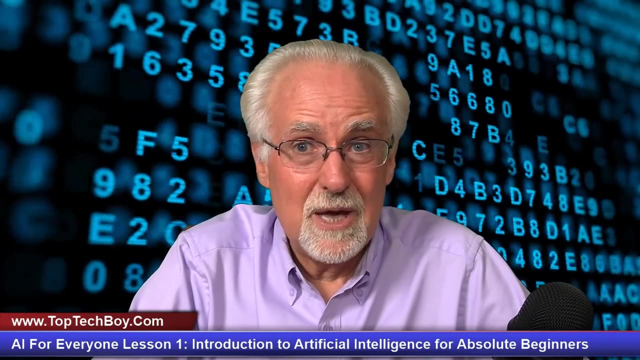 Linux and on some Jetson Nanos and things like that, And most people didn't have the board, or most people didn't, And so this is going to be artificial intelligence for everyone, because almost everyone has a PC. Okay, if you guys have a Mac, you can probably follow along, but you're going to end up in 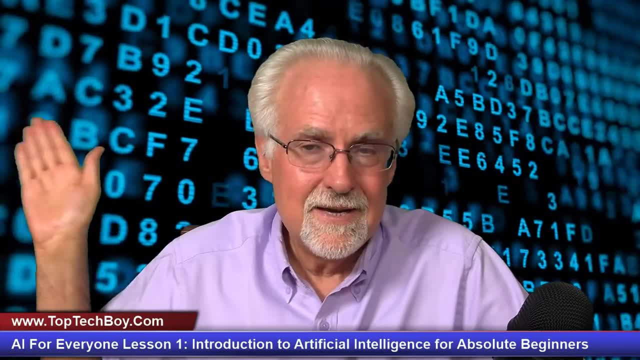 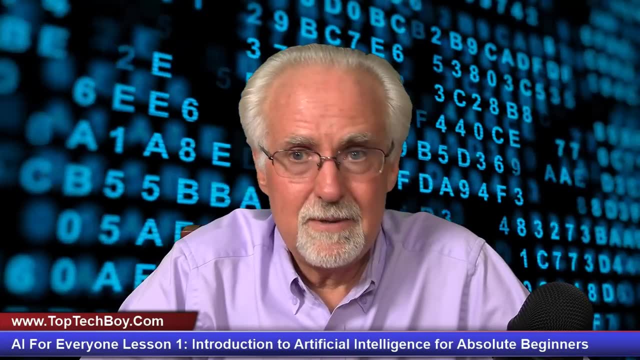 places that you've just got to figure things out because I can't make this series of lessons for all things to all people. So what do I say? Most people have a PC, and so I am going to be teaching this on the PC. Second thing: you're going to need, besides a PC, you're going to need a computer. 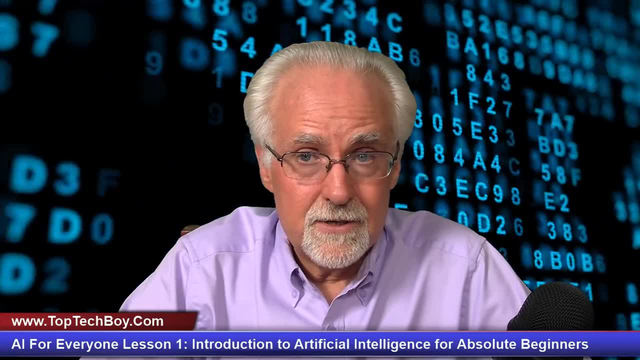 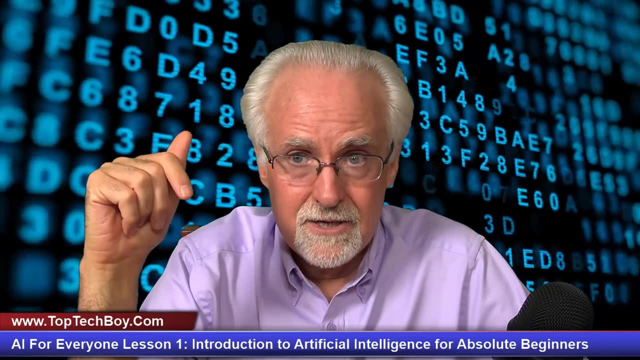 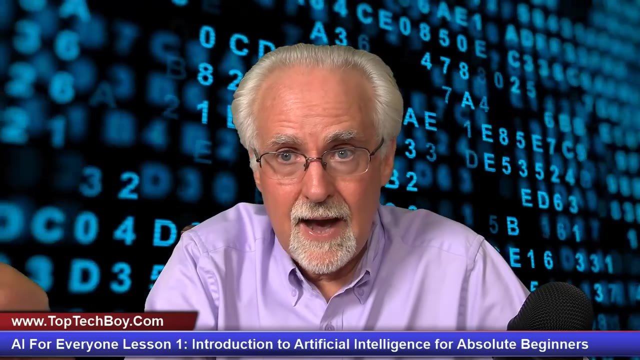 A webcam. I would suggest that your life is going to be much easier and my life is going to be easier if we are running the same webcam. I have a Logitech webcam. I have a link down in the description below. If you get the same webcam that I have, you can be assured that when I give code. 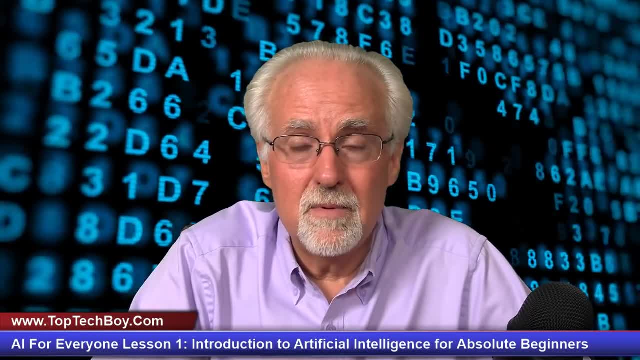 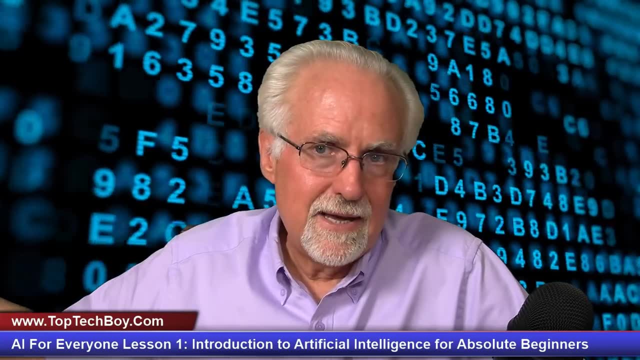 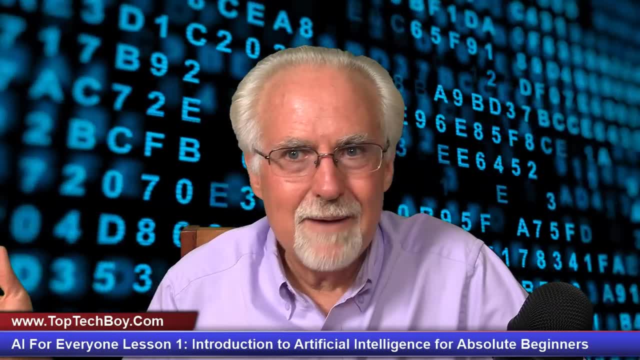 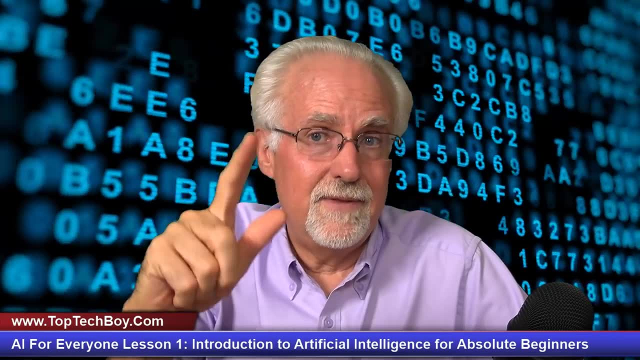 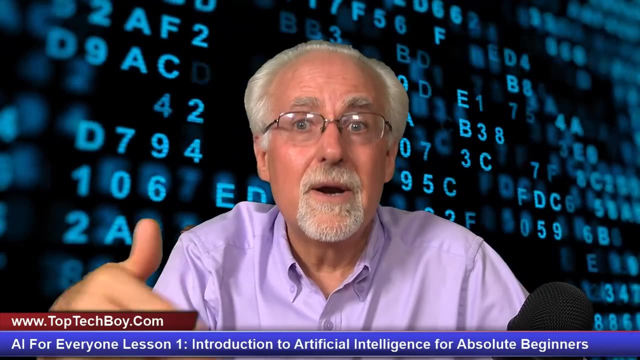 problem for you, right? I've got like 240,000 subscribers and I can't figure out every possible combination of hardware. So if you get the hardware that I have- this Logitech- look in the description down below- and a Windows PC running on Windows 10, we're going to be on the 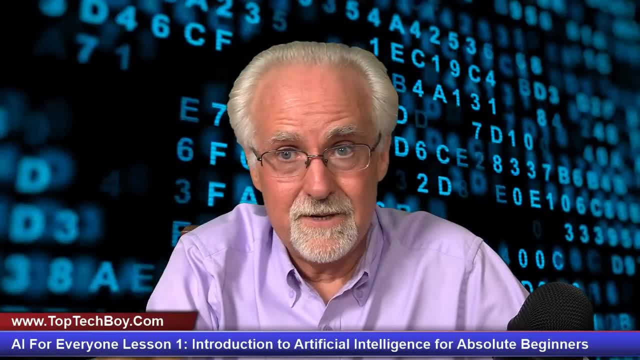 same system, and then we can focus on me teaching you artificial intelligence rather than us trying to figure out what's going on. So, if you get the same system, and then we can focus on me teaching you artificial intelligence rather than us trying to figure out why your webcam isn't working, Does? 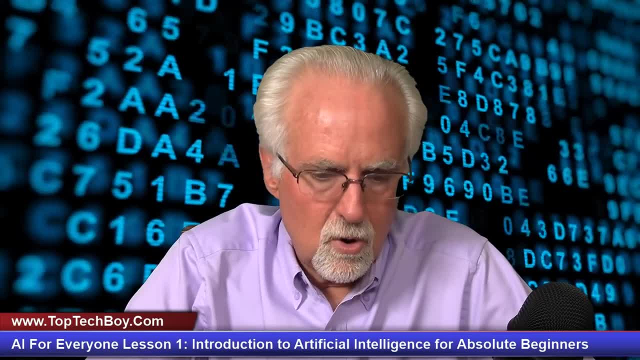 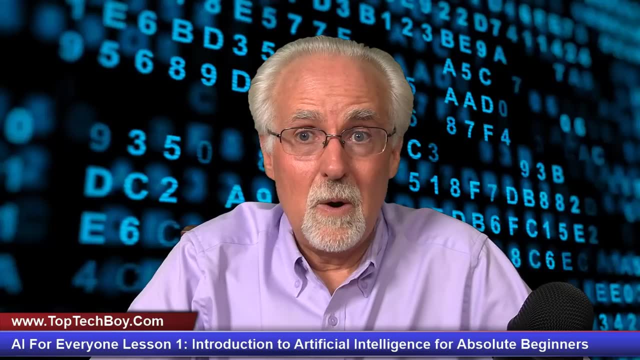 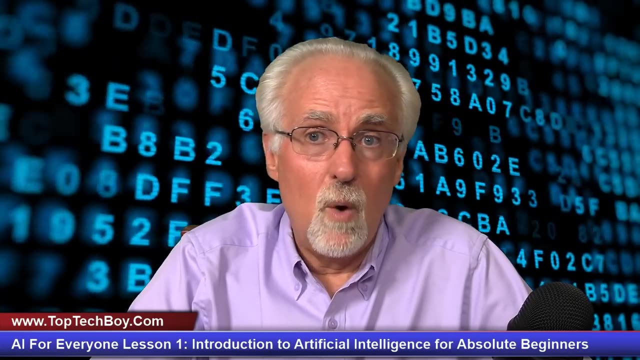 that make sense? Okay, I hope it does. Now, what approach am I going to be taking on this? I'm going to be taking an approach where, basically, you know you're going to understand it and it's going to be fun because I'm going to start with, we are going to be running on Python, And why? 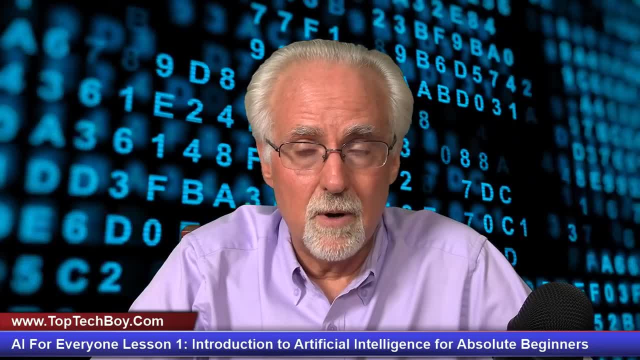 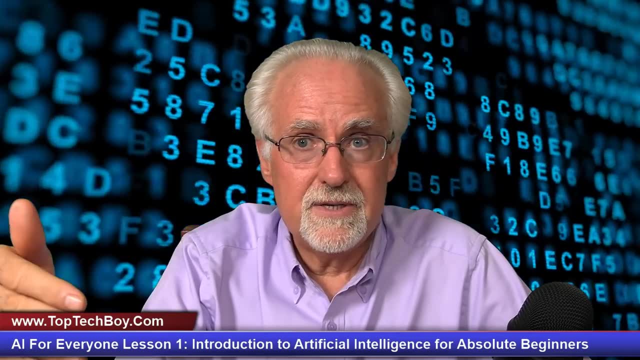 Python, Because Python is one of the most popular computer programming languages. I've already taught an entire series of classes on Python, And so Python is going to be one of the most popular computer programming languages, And so Python is something that most people are familiar with, And 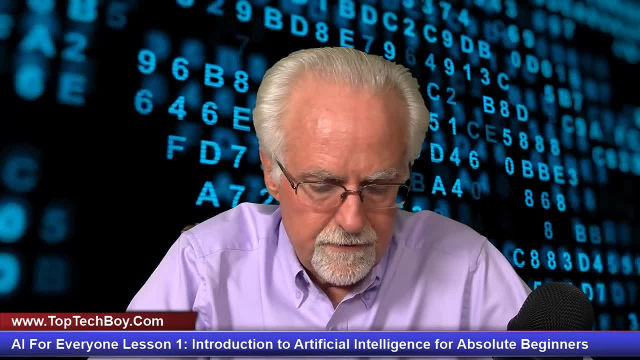 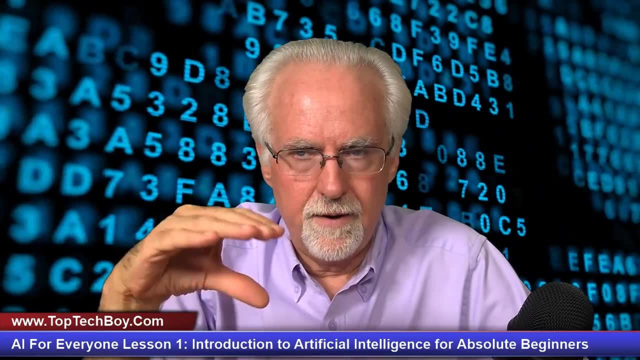 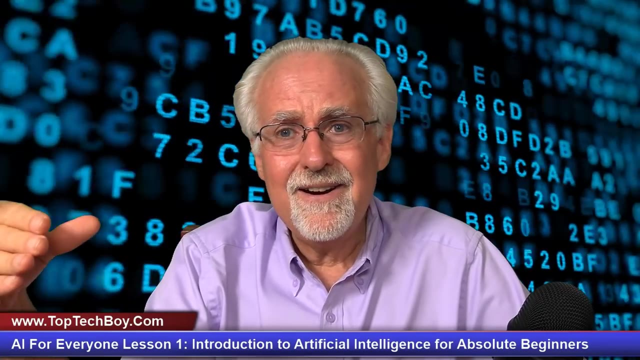 if you're not familiar with it, it's very easy to pick up. Now, one of the frustrations I had. another frustration I had as I was learning artificial intelligence. I felt like a lot of these platforms are trying to push you into their proprietary frameworks And there you're not. 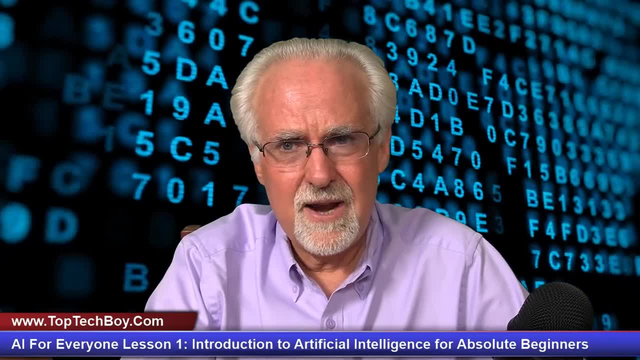 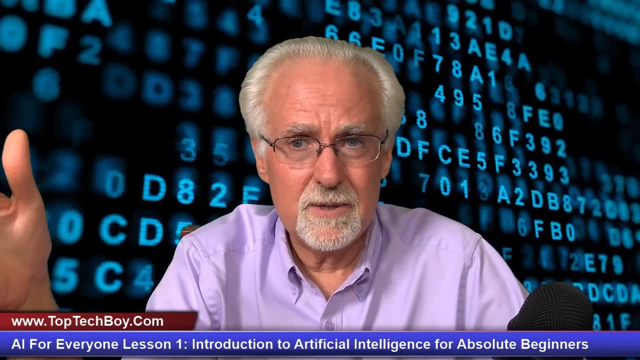 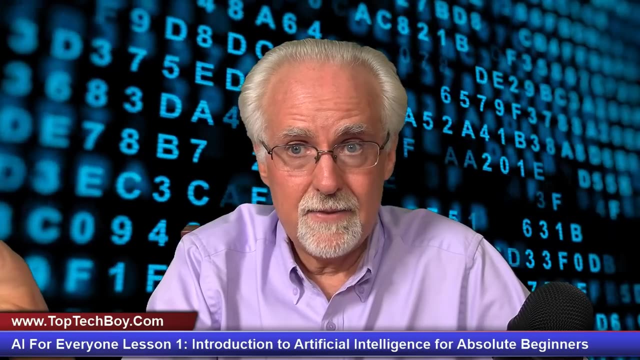 really so much learning artificial intelligence as you're learning their framework, And then by the time you learn the framework it's already changed and stuff like that, And so I'm going to be using very mainstream programming languages, language which is Python, and then very 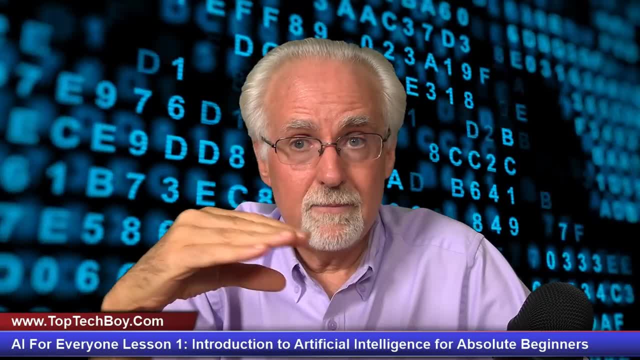 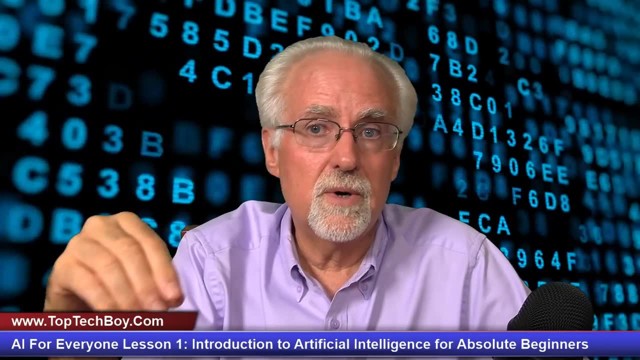 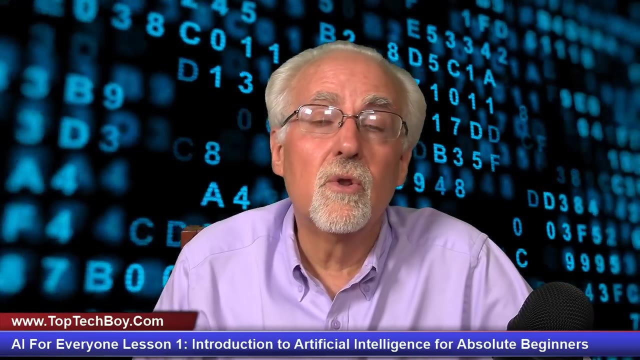 mainstream libraries, And the library that I'm going to be using with Python is OpenCV. Why OpenCV? Because it's open source, it's free. I'll show you in a future lesson how to download and install it, And then I'll show you how to use that, And then you're learning something that. 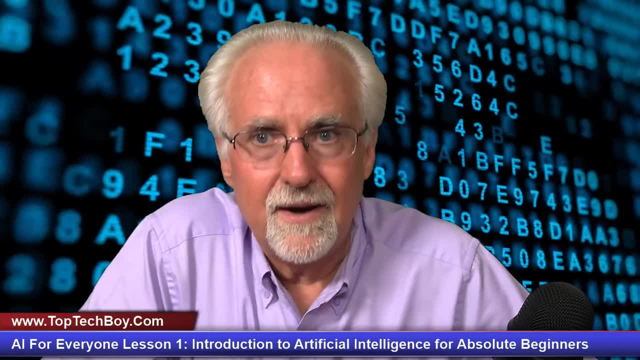 is a standard, and then you're learning something that is a standard, and then you're learning something that is a standard as opposed to learning, you know, like a proprietary system with NVIDIA or a proprietary system with Google or something like that. I'm going to be sort of. 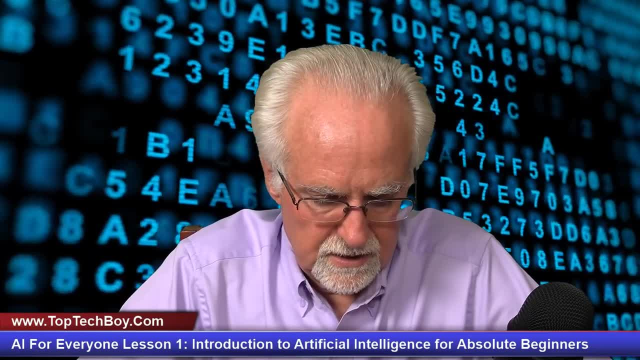 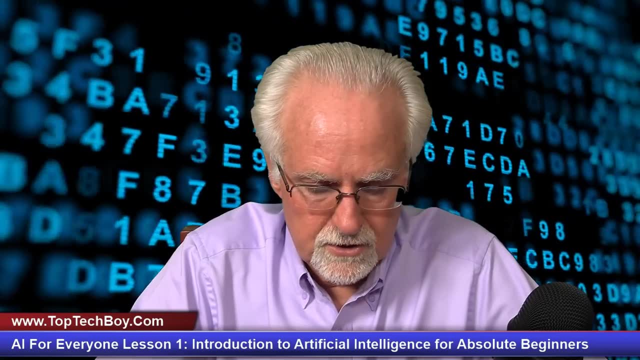 showing you a very mainstream way to do this stuff. So it's going to be Python based. it's going to be PC based. The library that's going to be doing the heavy lifting for us is going to be OpenCV. Okay, now, what I'm going to teach you, then, is I'm going to teach you how to use. 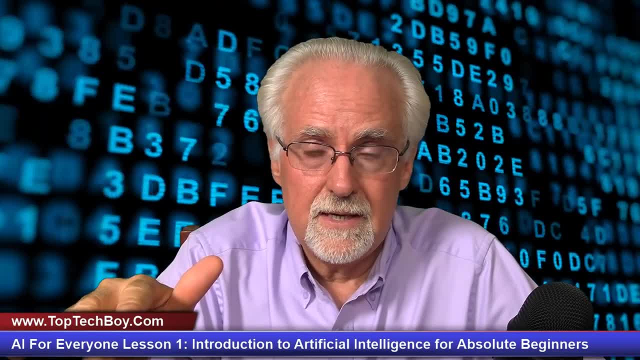 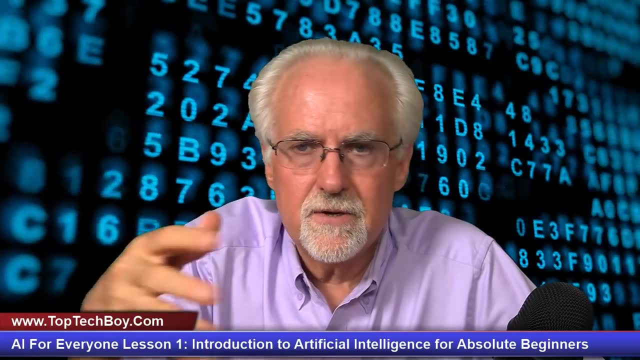 pre-trained models in OpenCV. Now I know a lot of people were saying: no, we want to develop. we want to develop the deep neural network from scratch. teach us TensorFlow. teach us how to do that stuff. Okay, if I started. 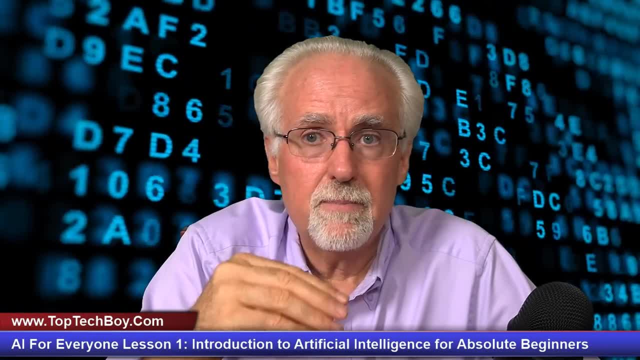 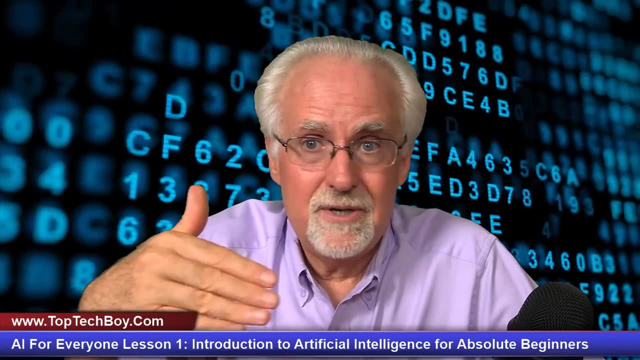 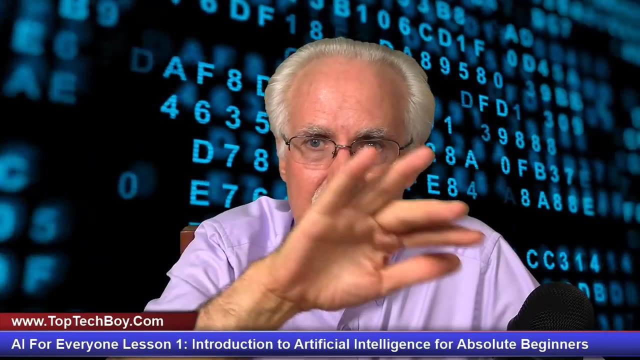 all the way back to starting with a blank sheet of paper and training a deep neural network from scratch, which I could show you how to do. it would take us like 50 lessons and we would be to the point that we would have the digits zero through nine and then it could look at digits zero through. 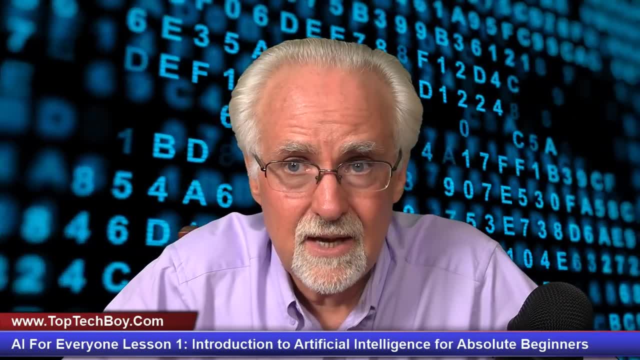 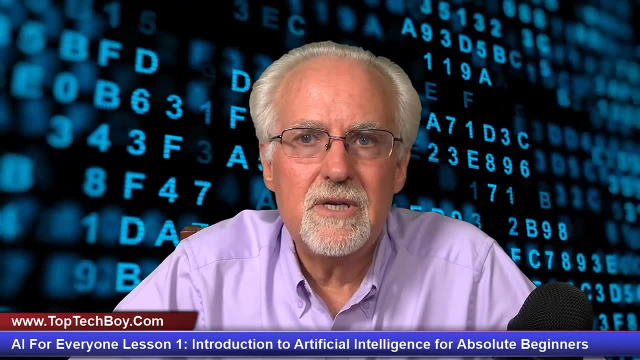 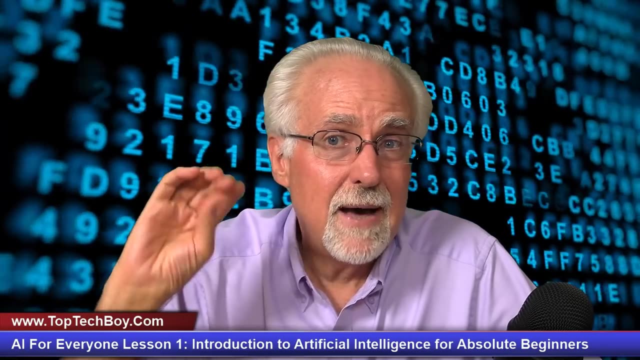 nine and it could recognize it. Now that is an interesting intellectual exercise and maybe someday I will teach you how to do that. But the problem is it's just so much abstract learning before you actually get it to do anything, or do anything interesting, I think, by about lesson. 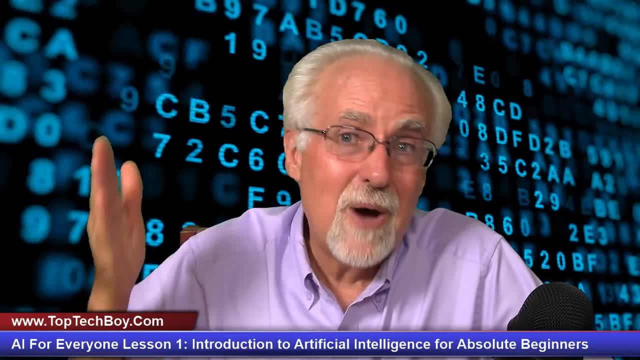 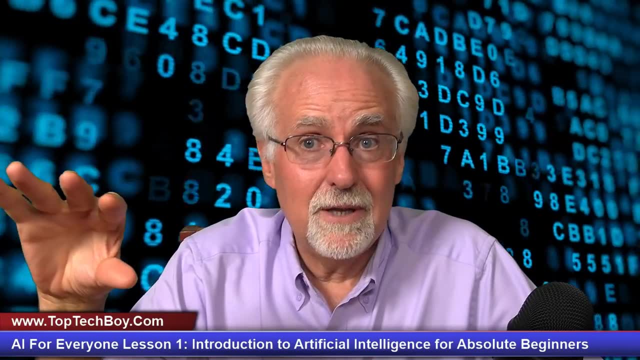 three. there would be four of you that would be still in the class. So I want to get us to the point that we're doing really cool and fun stuff as fast as possible. Now it is going to take us a couple of lessons that I have to do, but I'm going to teach you how to do it, So I'm going to 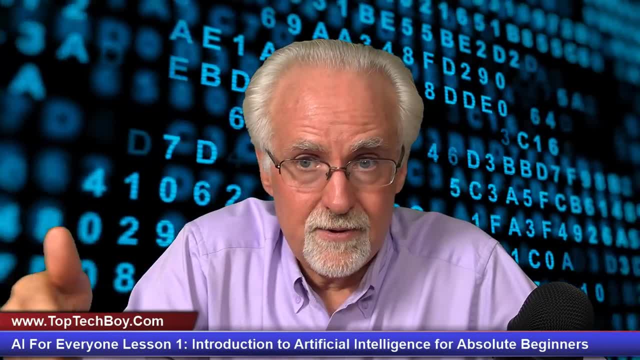 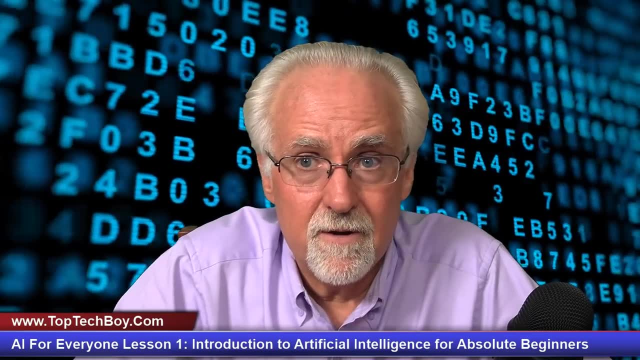 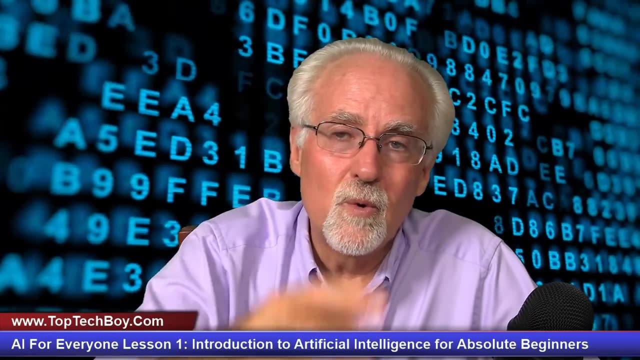 show you how to install the libraries and I show you how to install the packages. So just be patient, because I want to take you through that step by step. so you have an artificial intelligence computation platform on your computer that matches mine, and then we're really going to fly and we're 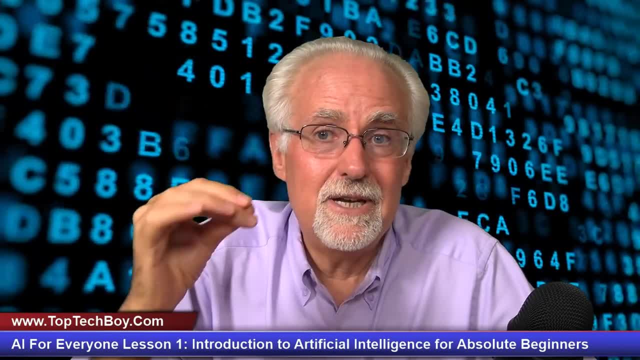 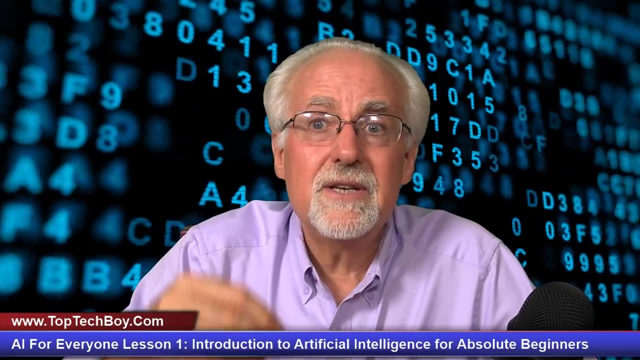 going to have a lot of fun, But I do need to take a little time to get you guys to get these packages installed, and that'll be the first couple of lessons. I'll show you how to do that, But what I'll show you then is I'll show you how to do it in a little bit. So I'm going to show you how to. 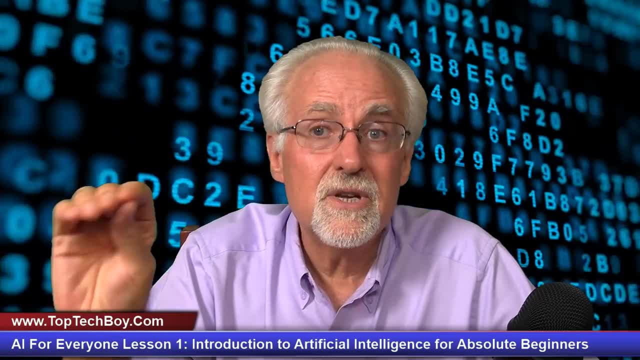 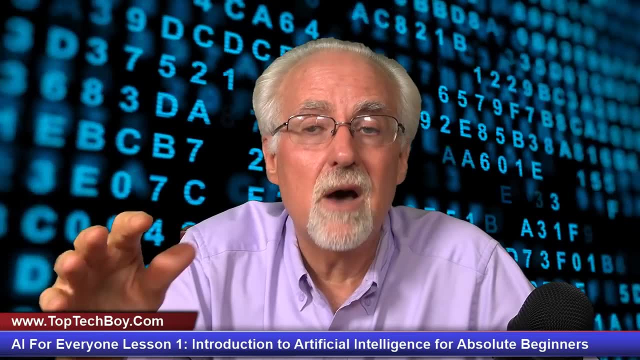 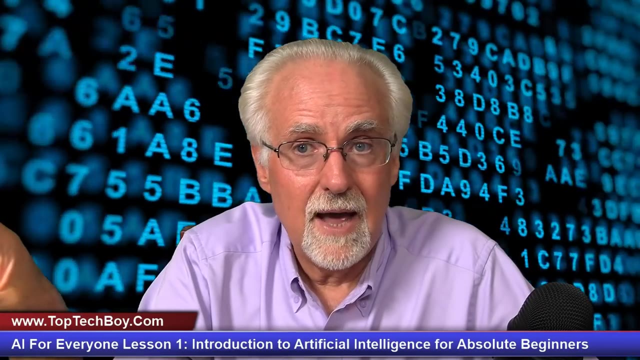 do it within OpenCV- how we can load pre-trained models and then we can get them to do really cool and really fun stuff. And then what we can do is we can take those pre-trained models and we can retrain them for things that we're interested in. So maybe there is a pre-trained model out there. 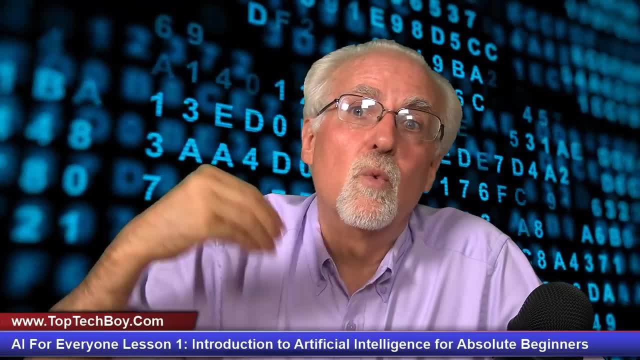 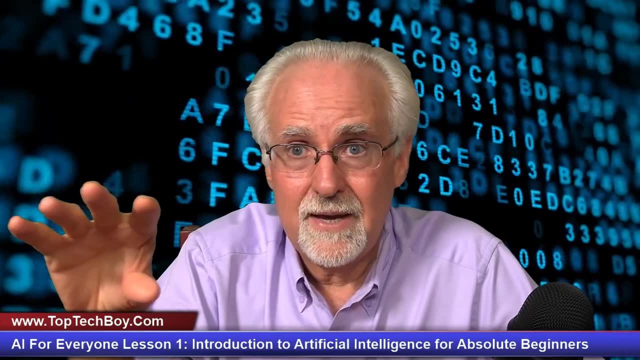 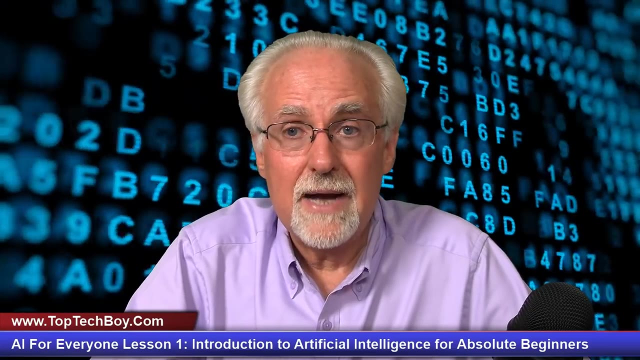 that can tell the difference between cats and dogs, but we retrain that model to tell the difference between a Raspberry Pi and an Arduino. Okay, but you see, we can do that by retraining an existing model, as opposed to trying to train a model from scratch. 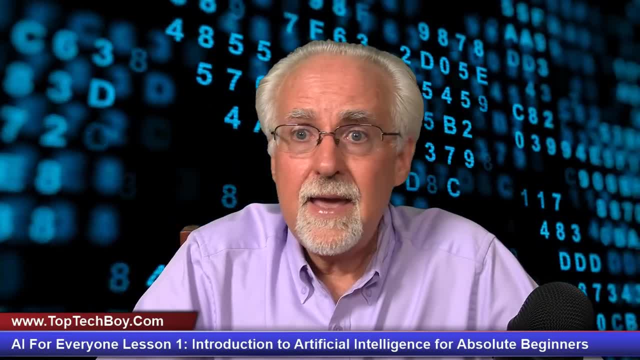 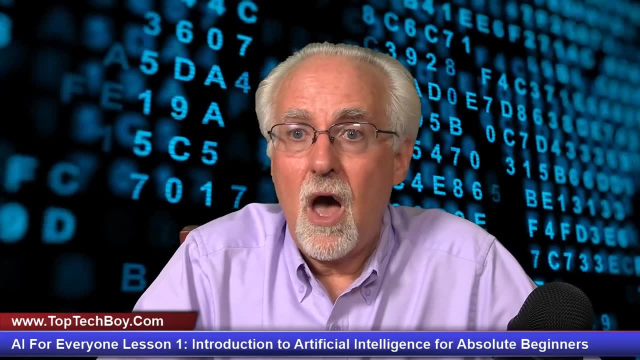 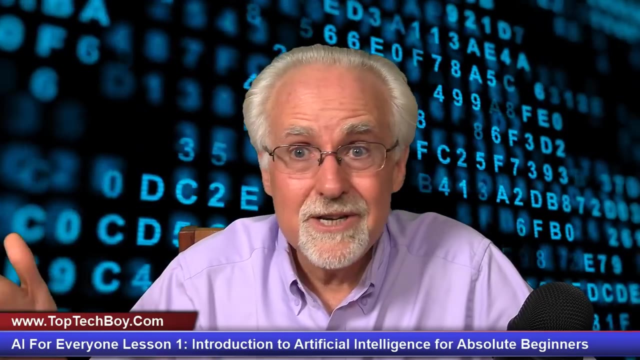 Now you've got to understand some of these libraries out there. they have trained these things based on millions and millions of images and hundreds of thousands of hours on these really huge parallel processors And we don't have the time or we don't have the money or we don't have. 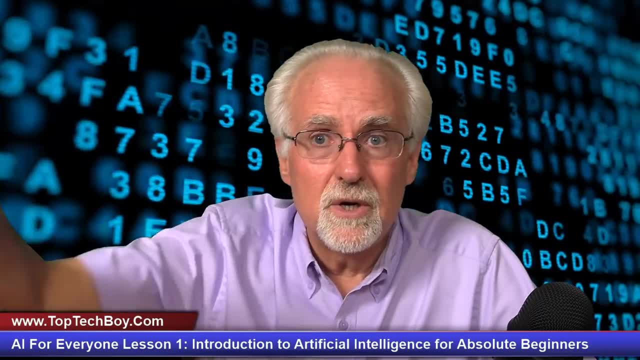 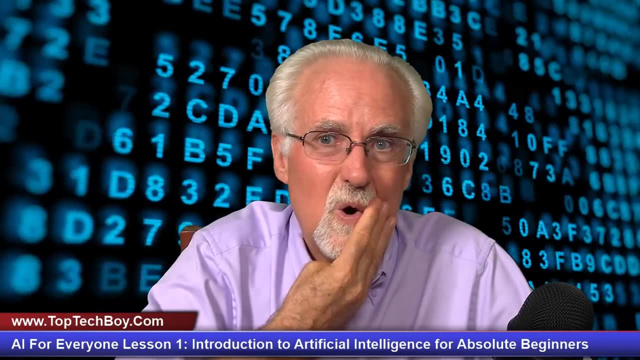 the resources to train these things ourselves. So we're going to take a little bit of time to get these things done ourselves, but we don't need to. We'll go grab one of those free ones. that's already been done, the heavy work done, and then we'll tweak it and we'll retrain it for what we 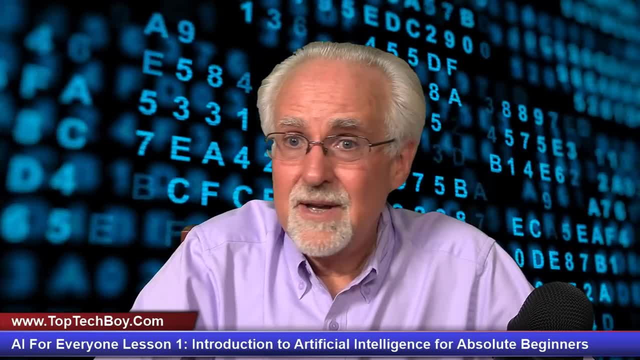 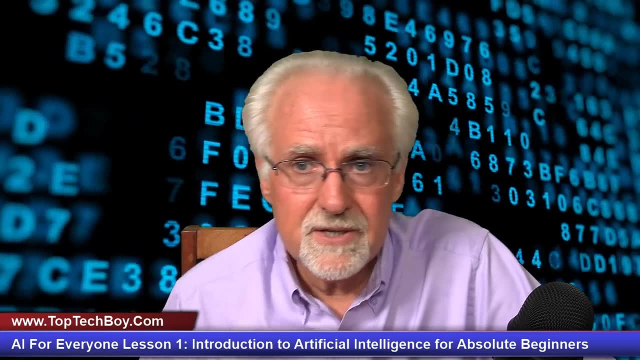 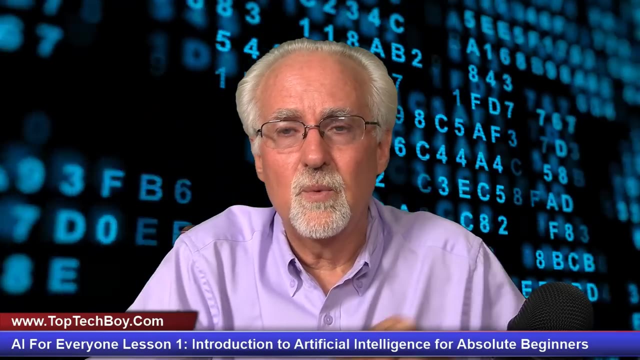 want. If we wanted to train something from scratch, man, it would take an incredible amount of computation power and an incredible amount of image processing and taking pictures and processing things, And it just turns out to be not that much fun. So we're not going to try to reinvent the. 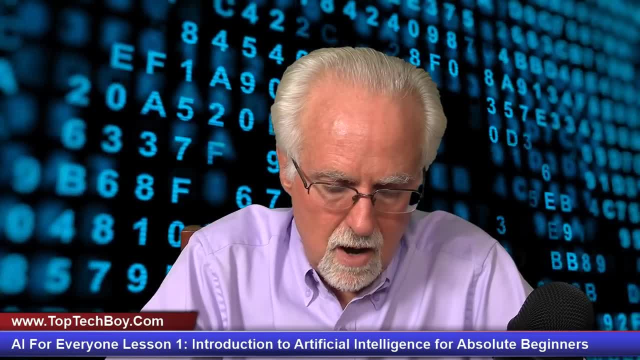 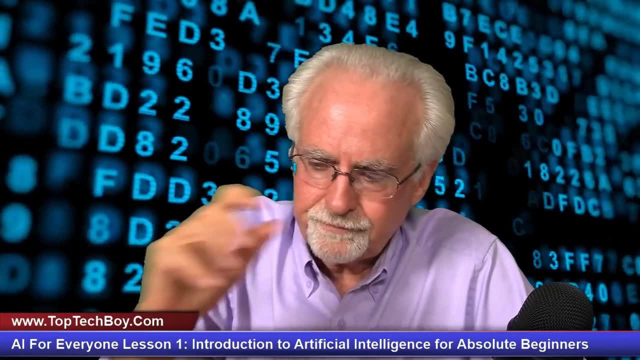 wheel We're going to be using as a starting point. we're going to be using as a starting point, we're going to be using as a starting point models that already exist. Okay, Then, what the really fun thing is: remember, excuse me, in our lessons, in our Python lessons. what have I taught you already? 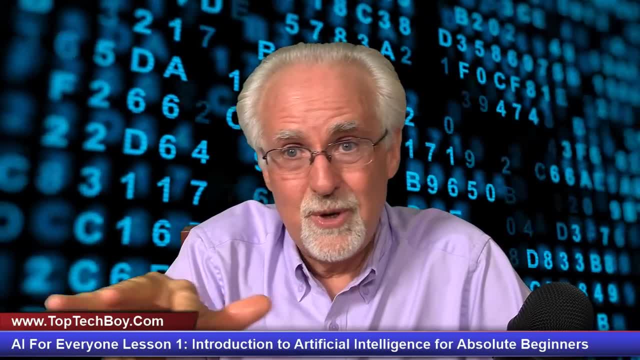 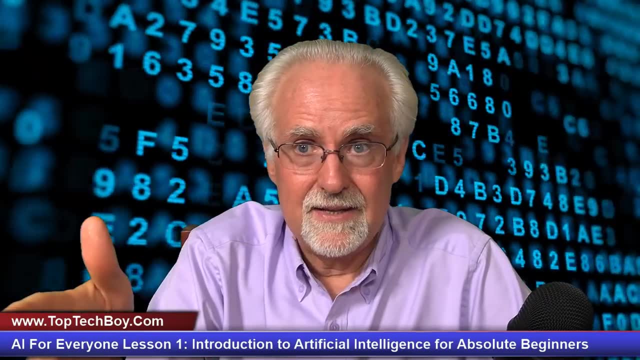 You guys that have been with me a while, I've taught you Arduino. Arduino is really fun to work with things in the real world, Like it gets data from sensors and then it sends commands to like actuators, servos, stepper motors. 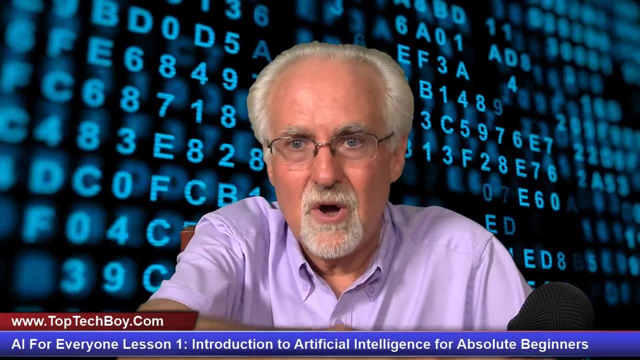 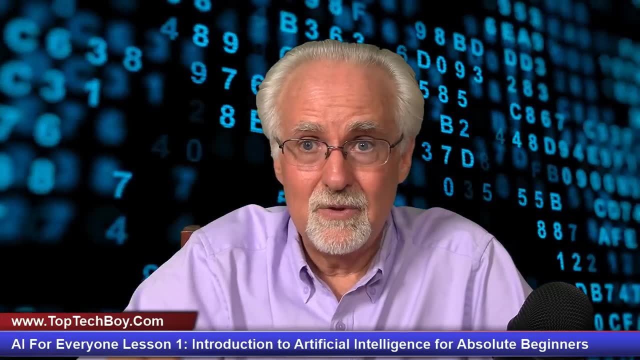 So you know LEDs, relays, And so there's all these things the Arduino can get data from. And then there's all these things that Arduino can make happen in the real world And that's a lot of fun. but the Arduino is very simple. You'd never be able to do artificial intelligence on. 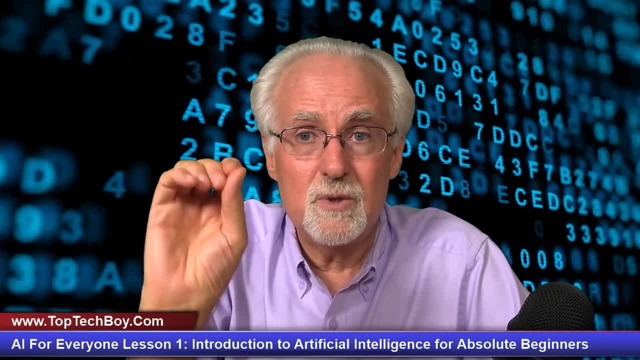 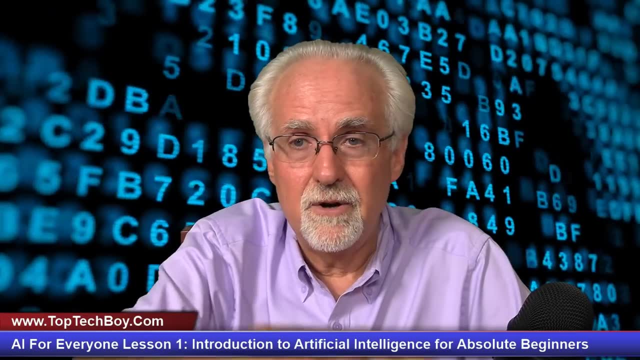 it. But in Python, in those Python lessons, what we did is we learned Python, which is very powerful, runs on your PC. Now we're working to get Python to work with the Arduino. And now, in this series of lessons, what we're going to do is we're going to work with the Arduino and we're going to work. 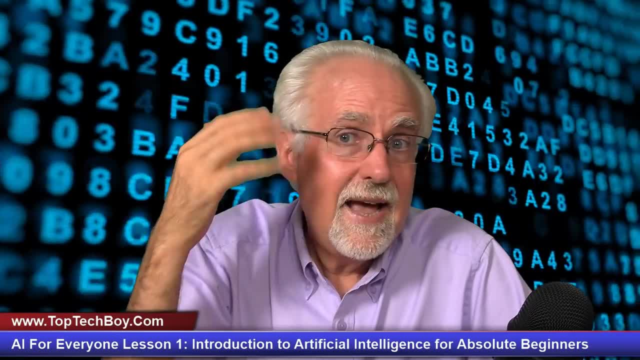 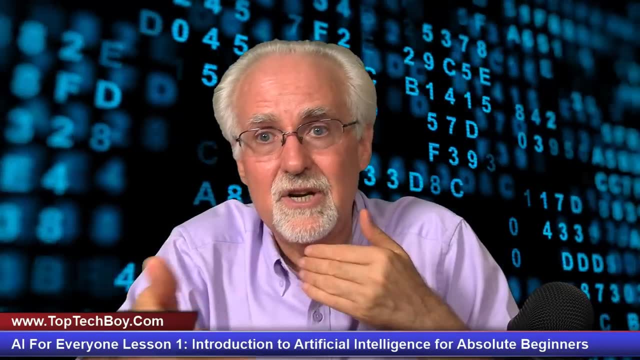 with the Arduino. So what I'm going to do is I'm going to show you how to do artificial intelligence And then what my vision is. it's going to be really, really fun, because Python is going to be doing artificial intelligence and it's going to be sending commands and data and information back. 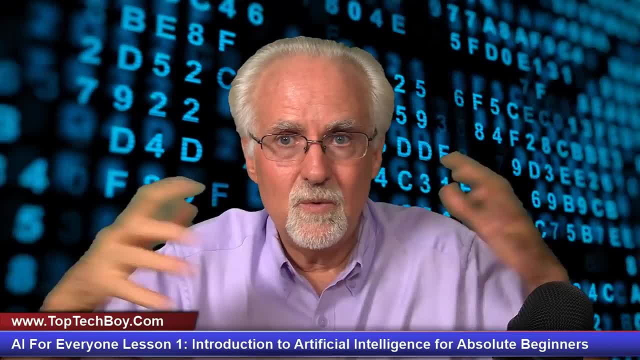 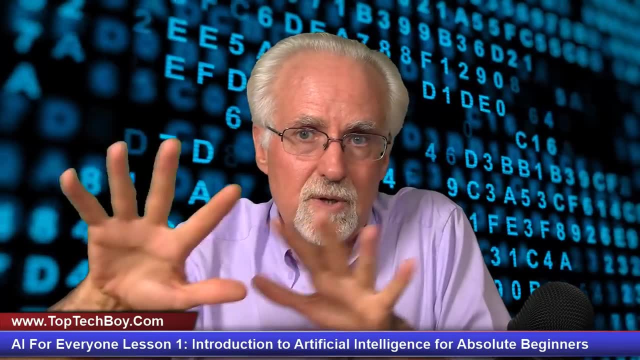 and forth with Arduino, And then Arduino is interacting with the real world, And so Arduino is getting data from the world, It's sending it to Python, Python is doing artificial intelligence and then sending commands back to Arduino, And so all of this is going to be really, really fun. 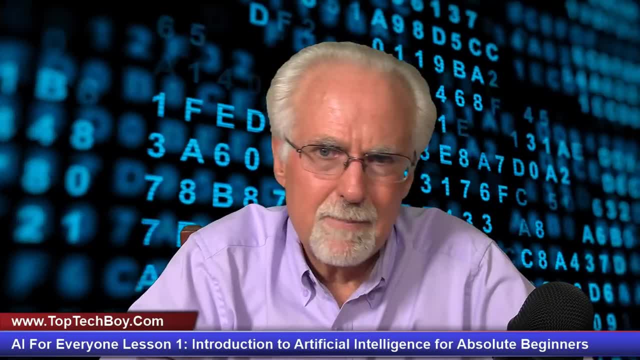 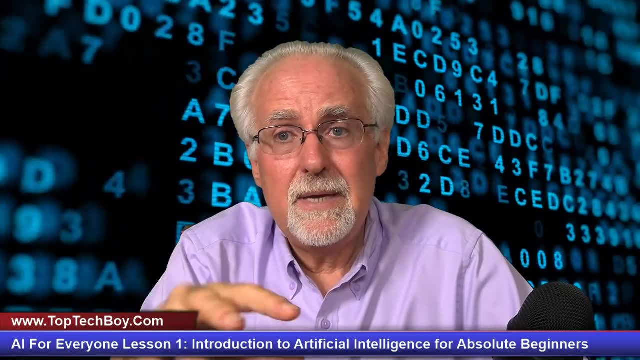 And so, all of a sudden, this real magic is going to happen, And maybe I'll kind of give you an example here of what I'm talking about. But our system is going to, in the end, be interacting with the real world. It's going to be getting information, getting data from the real world. 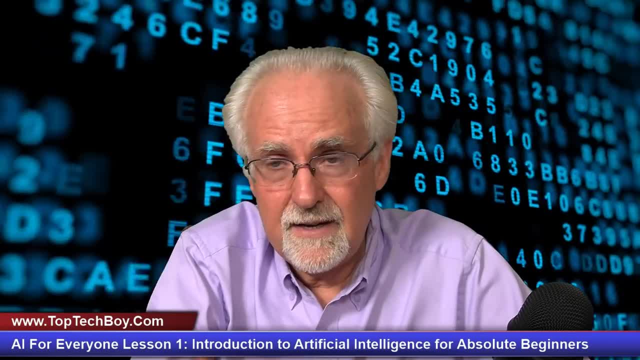 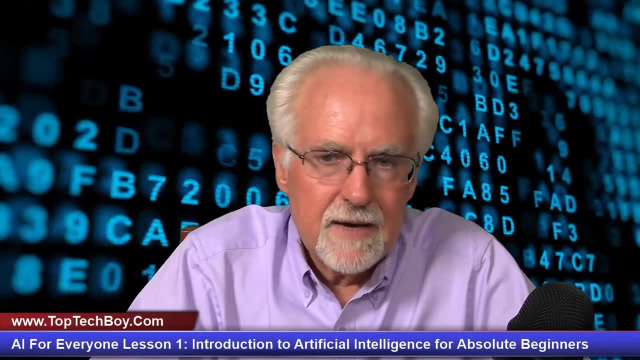 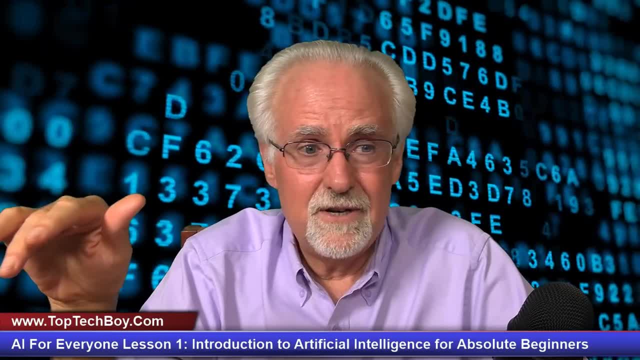 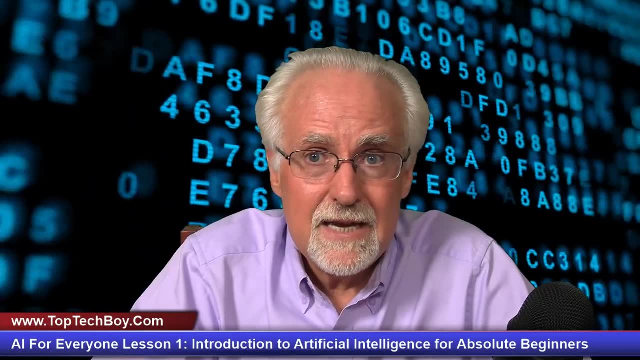 We're not coding today. I know you guys love to jump in and code, but I just felt like it was important for me to set the context for this class and for me to let you know what you're getting into and let you know whether this class would really be right for you or not. 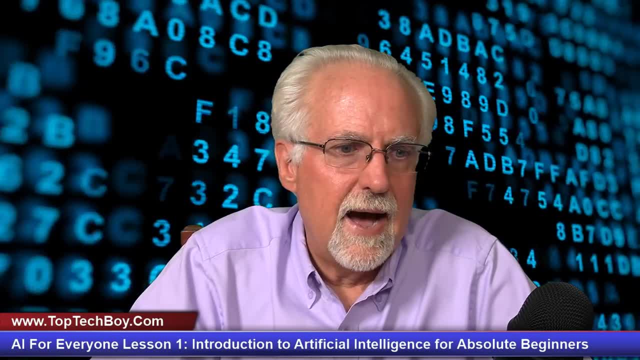 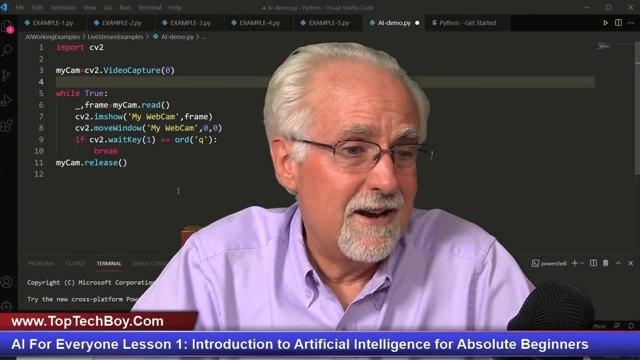 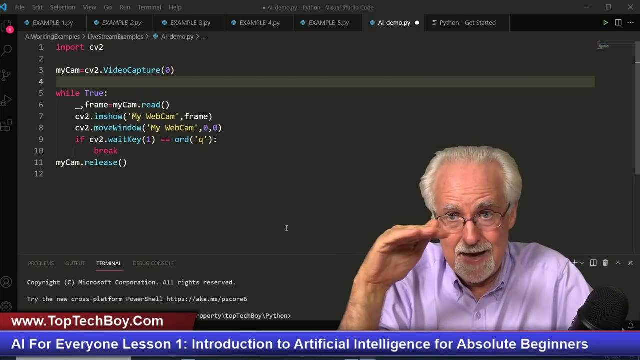 So what I'm going to do is I'm going to switch over here and I am going to show you sort of like one of the first things that we are going to be learning here, Like this would be kind of like the simplest OpenCV program. right, I said Python, So this is a Python interpreter, And 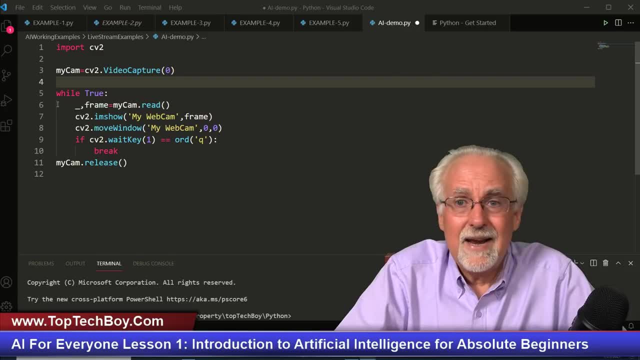 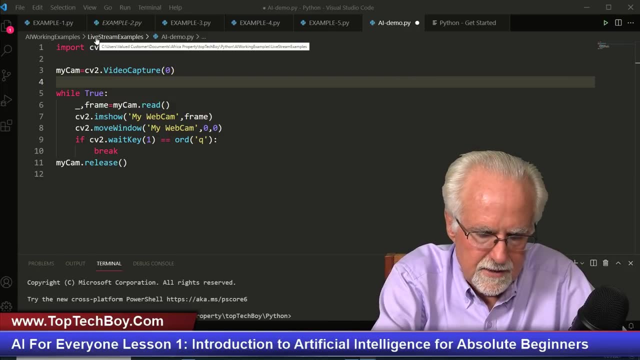 then I said we're going to be using the OpenCV library And I just want to show you just how simple some of this stuff is going to be. The first thing this program does: make sure that you can see it. Let me see if I can. That didn't work. That was an unexpected result. There it is. 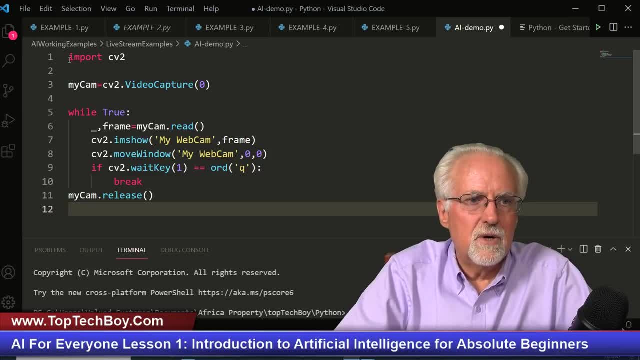 Okay, Hopefully you can see this a little bit better. So this is a Python program. I can import OpenCV. I then create a camera object that I called MyCam, And then I have a loop here. And what do I do in the loop? Well, I read from my camera object. I read from my camera object a. 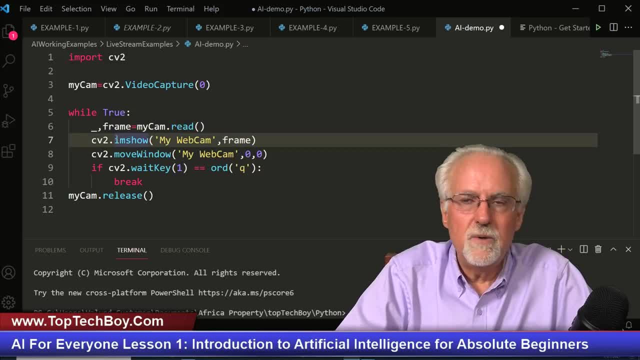 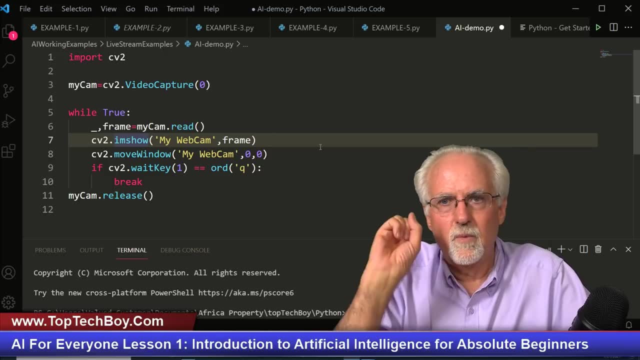 frame. Now I have one picture. Then what do I do? I then show that picture with the CV2.imShow, And so I read a frame. I show a frame, Read a frame. show a frame. Read a frame. show a frame. 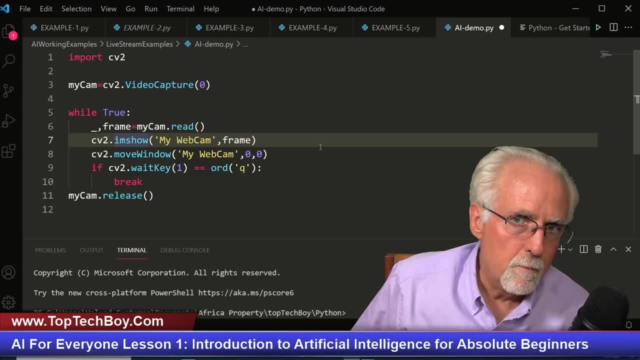 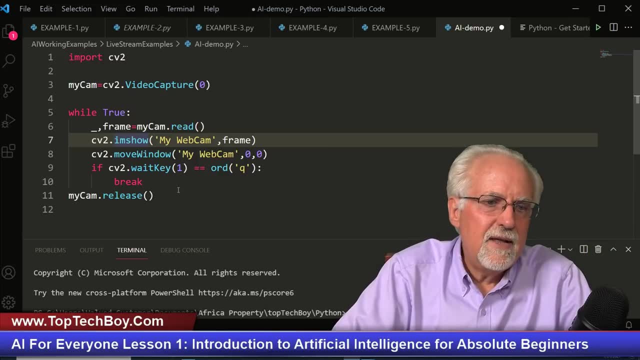 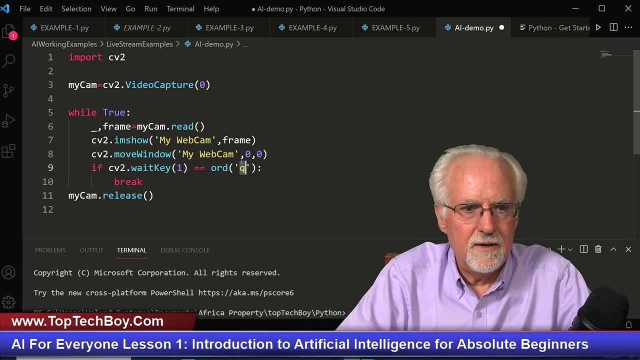 If I keep doing that, have a what? I have a movie, I have a video. so what this program does is it goes and grabs frames and shows frames and then I have a way to gracefully exit that. if the program sees the letter Q pressed, then it is going to quit and 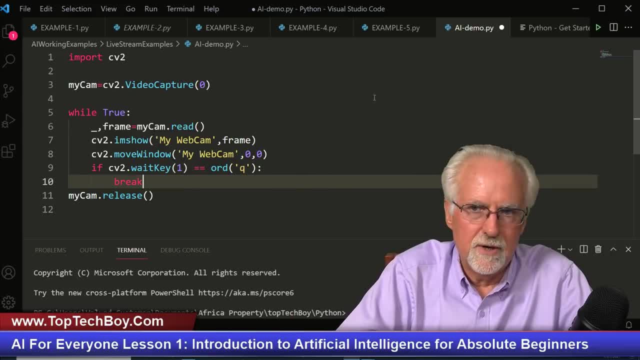 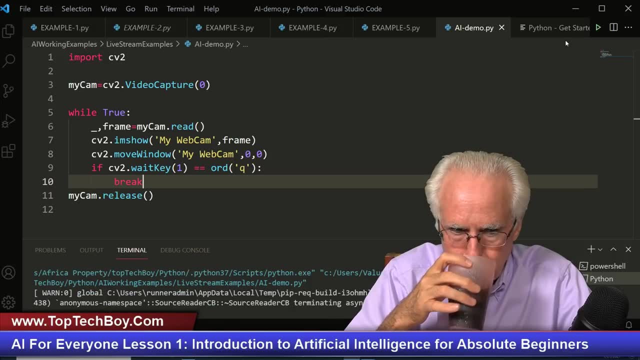 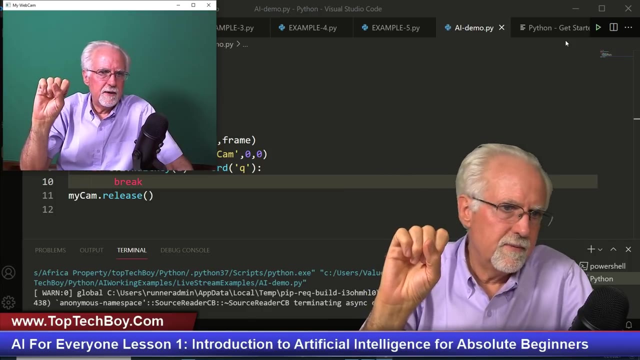 then it's going to release the camera back to be available for someone else. so if we run this program, it is ten lines of code, it's under ten lines of code actually. and boom, look at that, read, read a frame, show a frame. okay, now, why is it a little bit glitchy? it's a little bit glitchy because I am running. 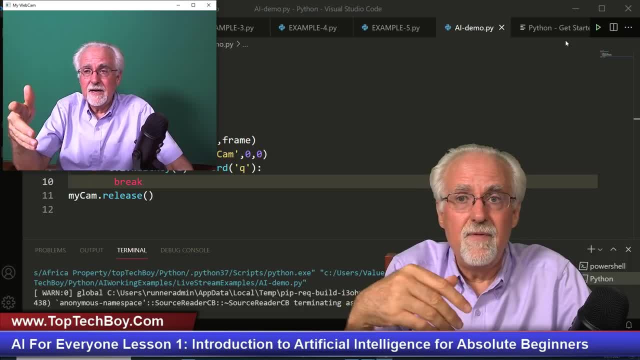 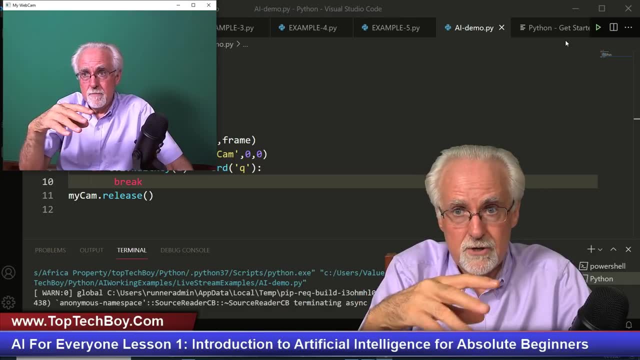 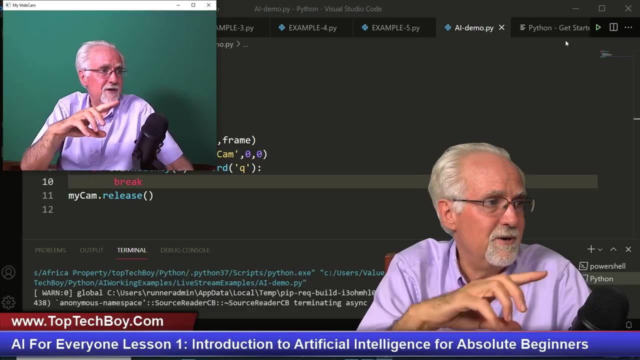 Wirecast to do this video recording and that is really, really really putting a huge load on my graphics card and on my computation. this will run much smoother and much faster for you if you're not trying to live stream you and do real-time video processing using using Wirecast. so the reason it's a tad. 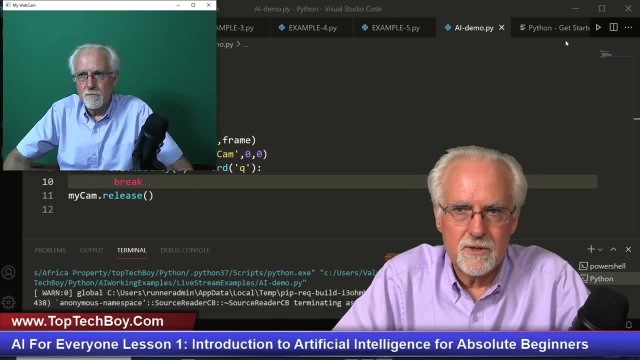 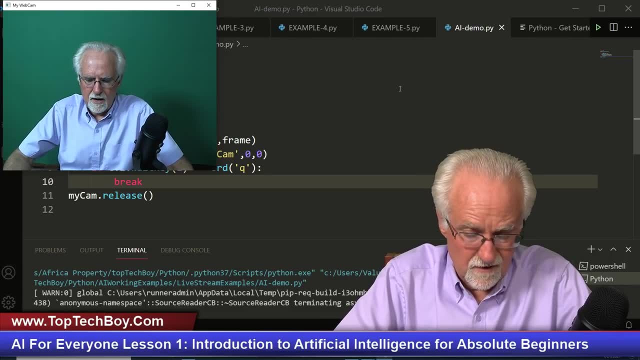 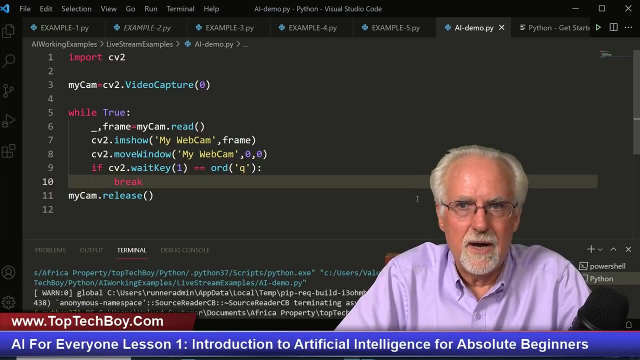 bit glitchy is because I have a huge monster load on my CPU and on my graphics card running this, this video processing software, so that you can have this lesson. but I digress, okay, so now remember, if I click Q it makes it go away. so now, was there anything artificial? 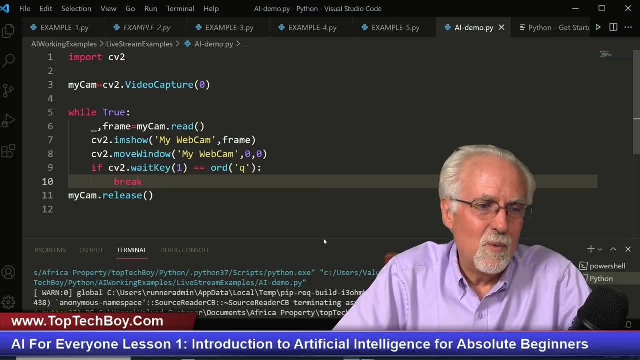 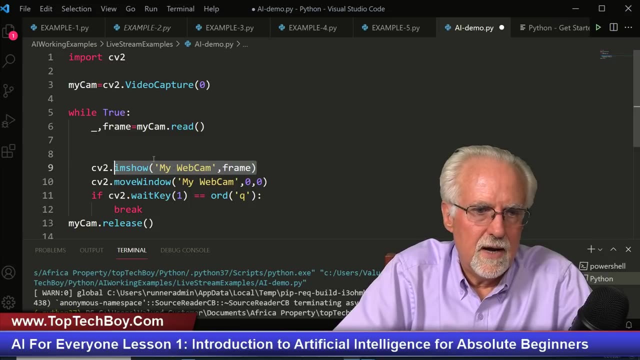 intelligent about that? no, but it is kind of cool that with under ten lines of code we can make our own little webcam program. now this is where the artificial intelligence comes in. you see that I read the frame. I read the frame here from the camera and then here I show the frame. so I read a frame, show a frame. 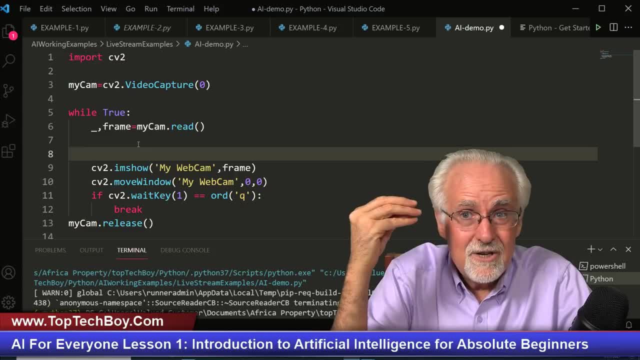 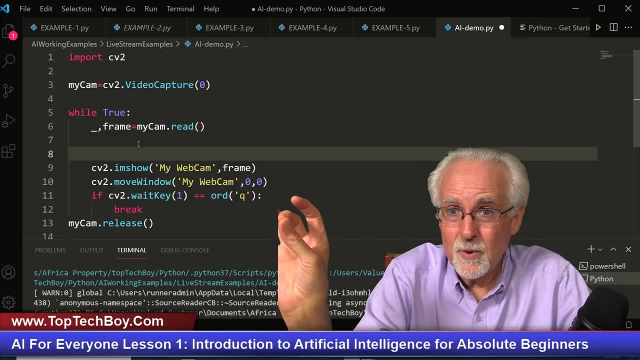 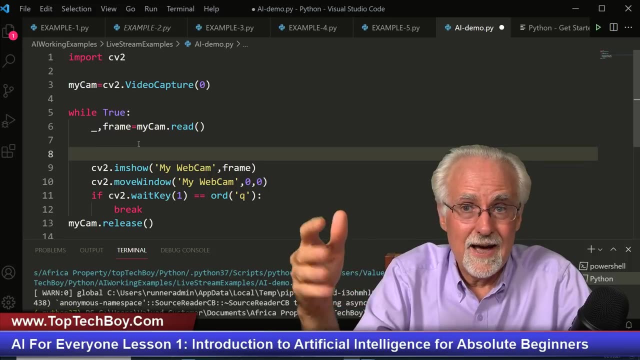 read a frame. show a frame. now, what I can do is I can come into this program between the read frame in the show frame and this is where the magic happens. this is where the mischief happens. I want you to think like you can run a video. real time is like 30 frames a second. 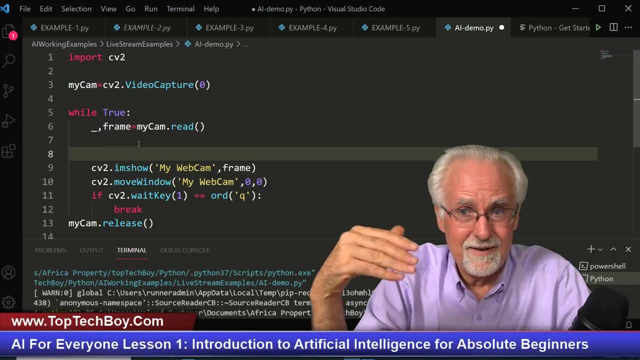 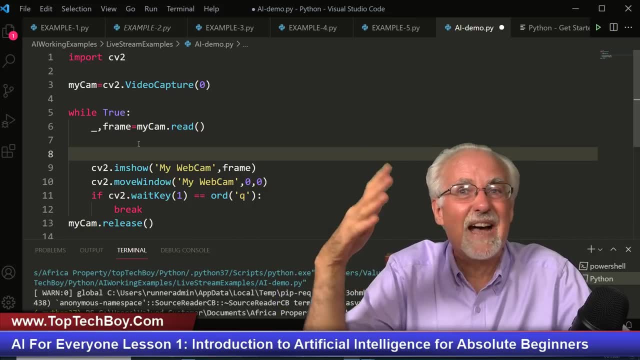 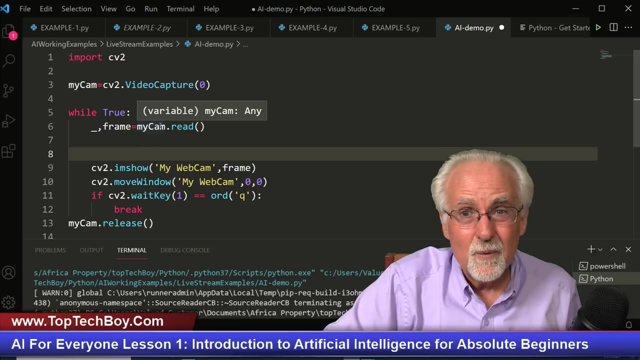 And so how much time do you have between read and show? You have like a 30th of a second, And for a modern graphics card and for a modern computer that's like infinite time. It's like you have all the time in the universe between the read frame and the show frame. 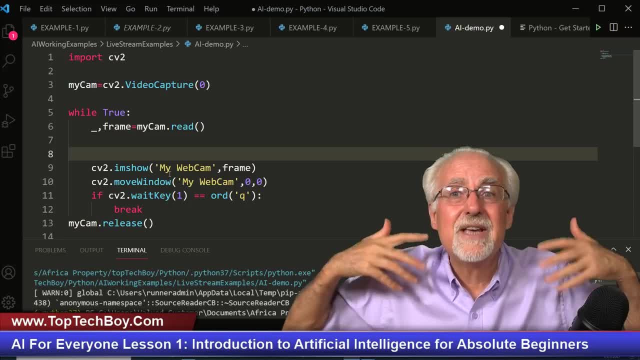 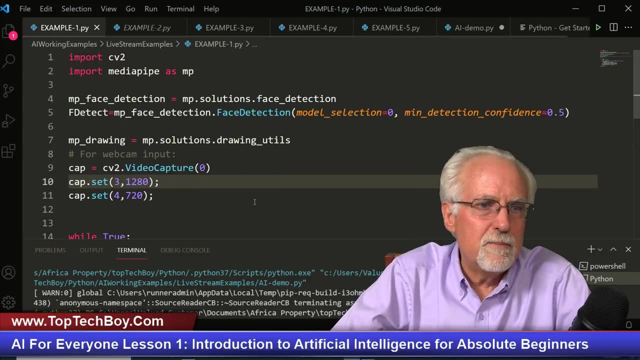 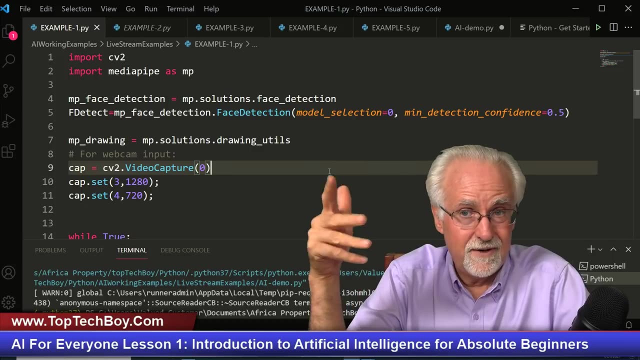 to do all of these really, really incredible things, And that is where the magic happens. That's where the artificial intelligence happens. So let's do a little bit more complicated program now, instead of just importing CV2.. In this particular example, I'm going to be showing you lots of different libraries and 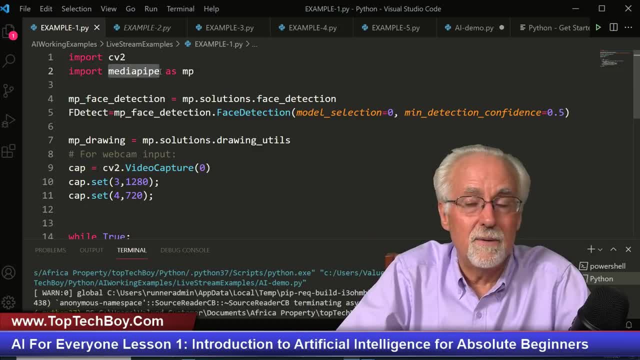 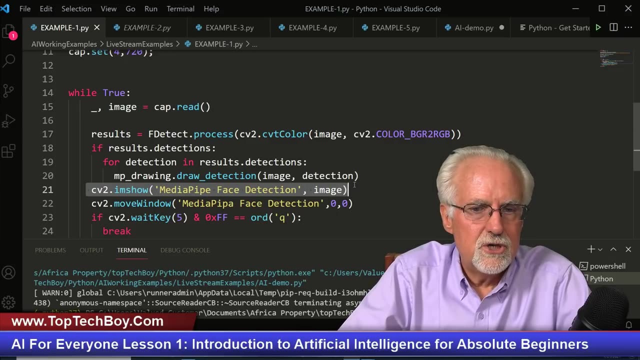 lots of different programs- I'm just happening to use a library called MediaPipe- which are some pre-trained artificial intelligence programs, And then what I am doing now is where was my loop? I still read, I read the frame and I still show the frame. but between read and show what I am going 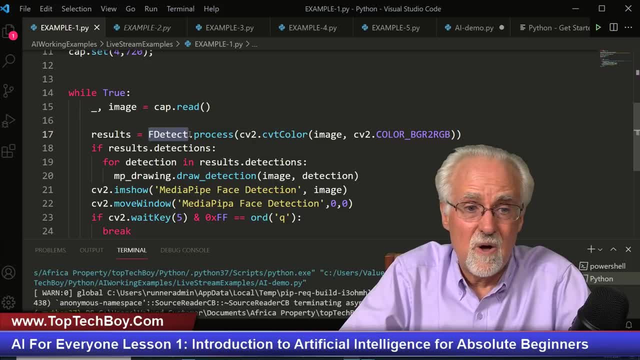 to do is: I am going to run a process called face detect, And so it takes that image and it processes that image to find the faces and then it gives you a result And then if any faces were found, then what it is going to do it is going to do is it's. 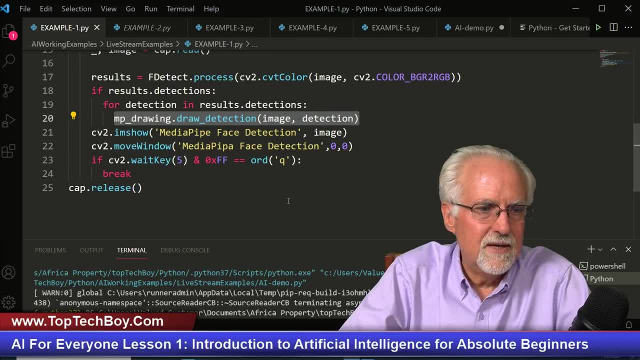 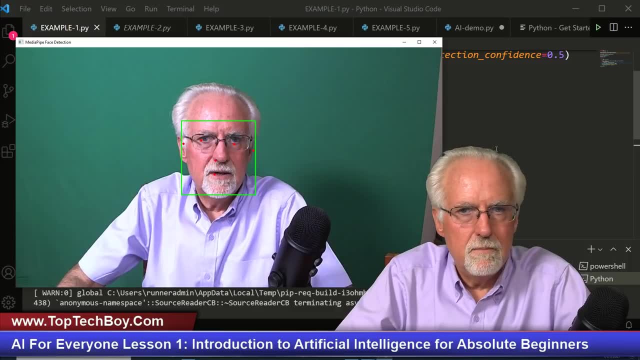 going to do some drawing on those faces, Okay, So still, I'm like under 25 lines of code And what I can do there is boom. what did I tell it to do? I told it to find and analyze the face. 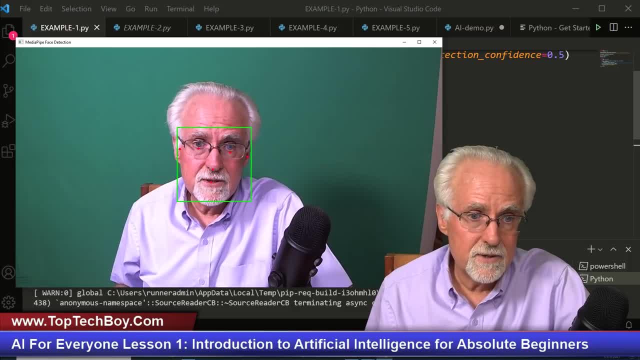 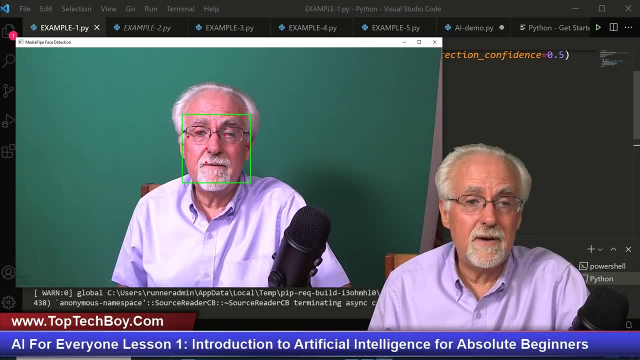 Now it drew a box around the face and then also look, it is saying, not only I have a face, not only the face is here, but look, I'm going to look at that face and I see two eyes. I see a nose. 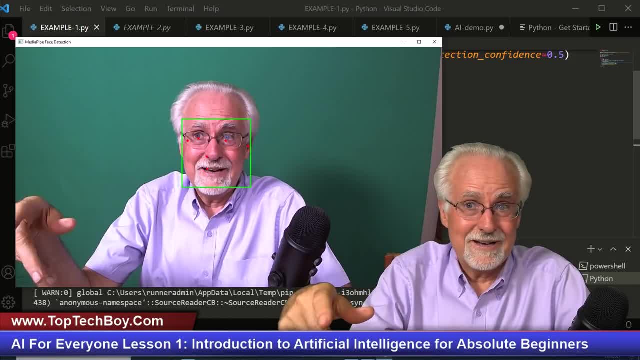 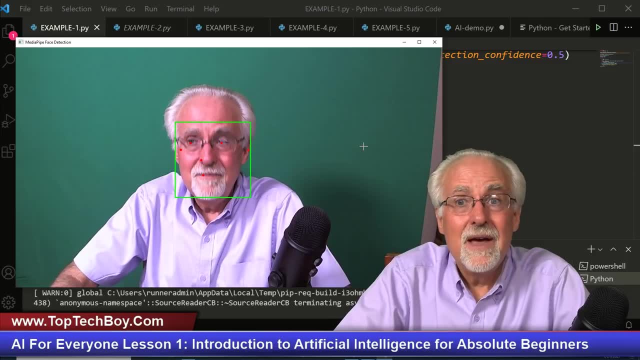 I see a And I see two ears. So all of a sudden I've got X, Y position of nose, eyes, mouth, ears, box in the face. Now, all of a sudden, this is kind of starting to be artificial intelligence. 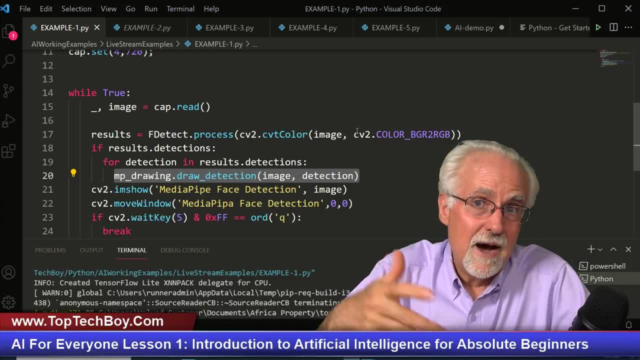 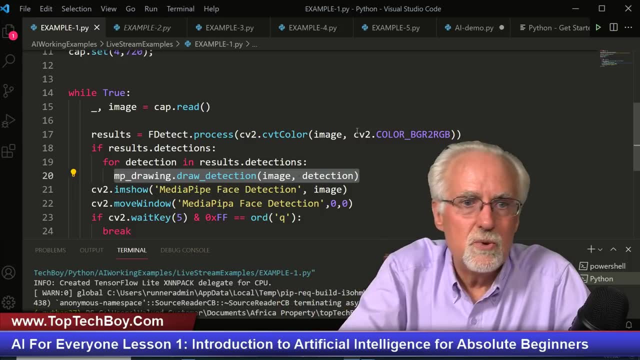 And that was just a few lines of code to let me do that. Now imagine that, based on that, I could start sending commands down to Arduino to do certain things. based on what you are seeing in the picture, I could do more sophisticated things. 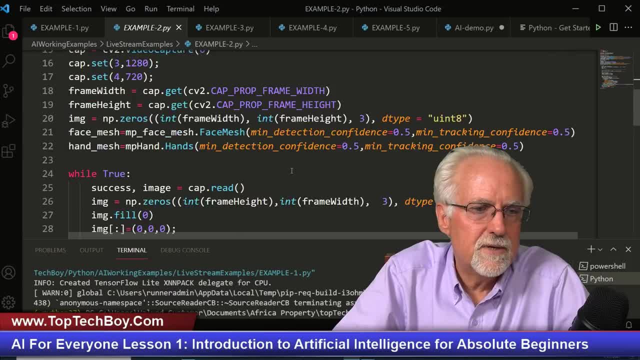 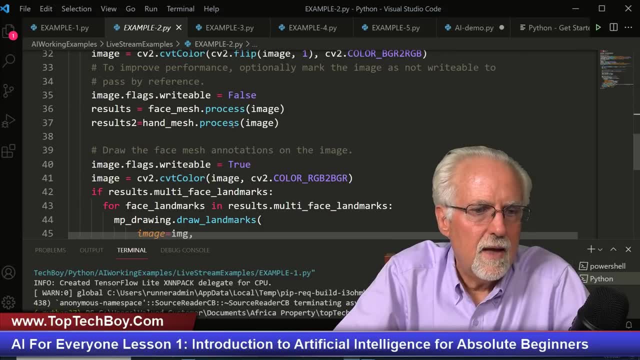 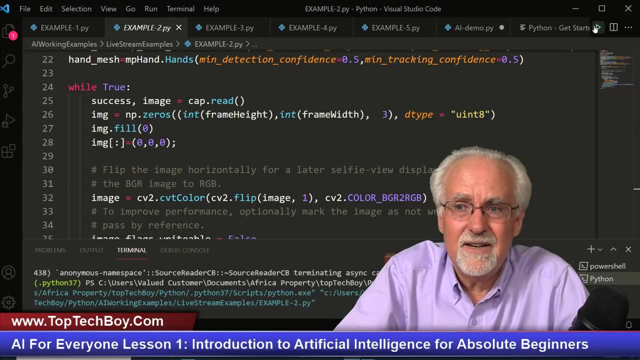 I could do more sophisticated things between- still we are, this is more lines of code you can see, but still, between the read the image here and the show the image here, I'm now doing some more sophisticated analysis And let's see where did it go. 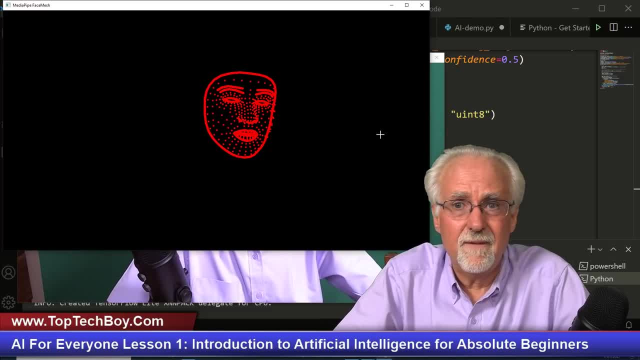 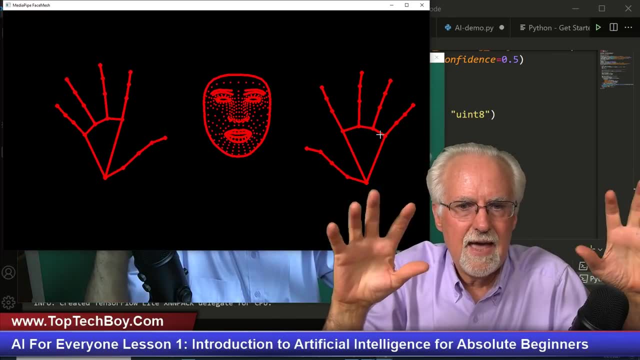 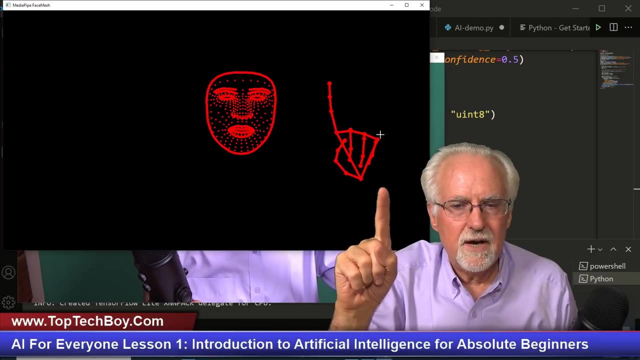 Okay, Here you can see that I'm not only detecting a face. I'm kind of trying finding facial landmarks and then look at this, I'm also finding the hands. Okay, So I'm finding hands and face. Now this point here, the tip of the finger. there I have an X- Y coordinate for the tip of that. 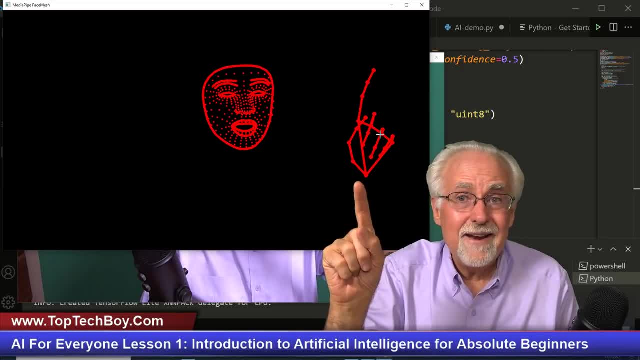 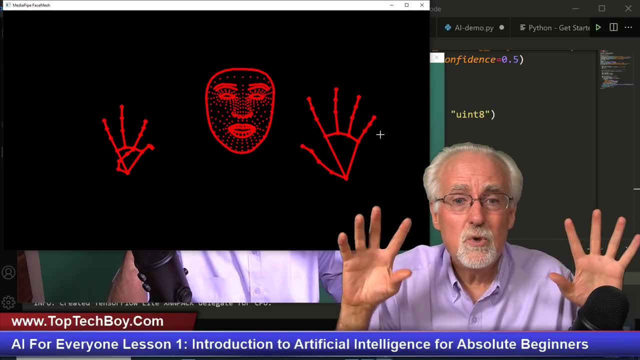 finger. I have an X- Y coordinate for the eye, So I know how far my finger is from my eye. I've taken this complex picture and I've reduced it down to math, And so now, all of a sudden, we could do something like say: 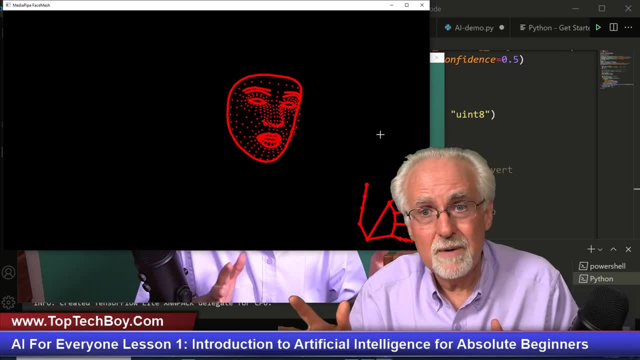 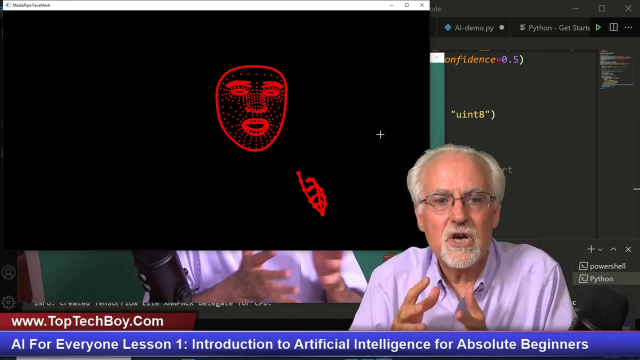 if my fingers started getting too close to my eye, beep warning me. Hey, don't touch your face. You know, we've got the virus thing going on out there. Don't touch your face. You see. see, all of a sudden you could start interacting with the world based on artificial intelligence. 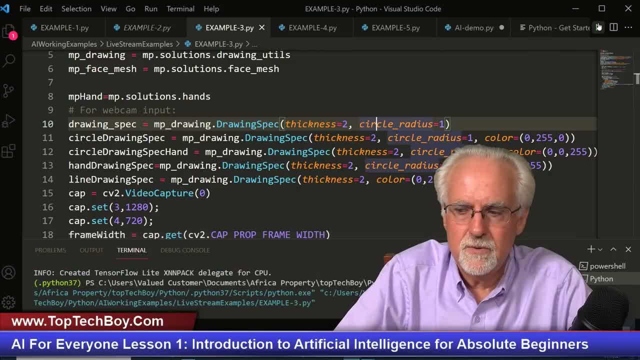 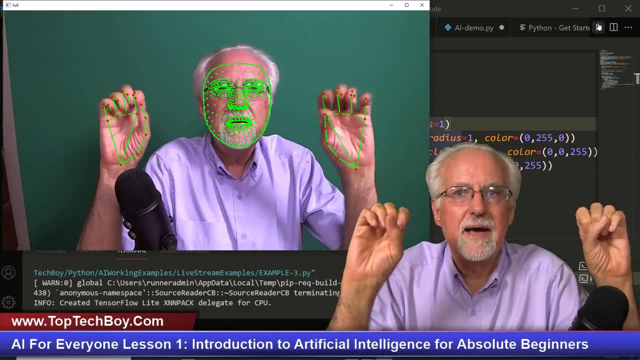 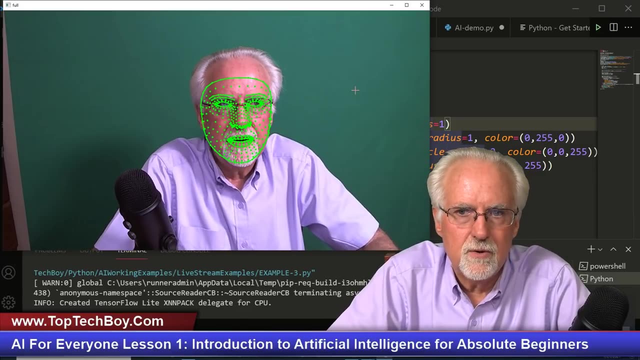 Okay, Let's do a couple more quick demos here. Let's see what this one does. Okay, Here, what you can see I'm doing is I can superimpose That analysis back on top of the original image, which is kind of cool. 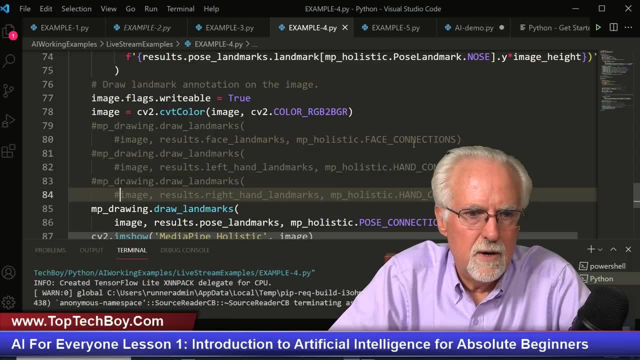 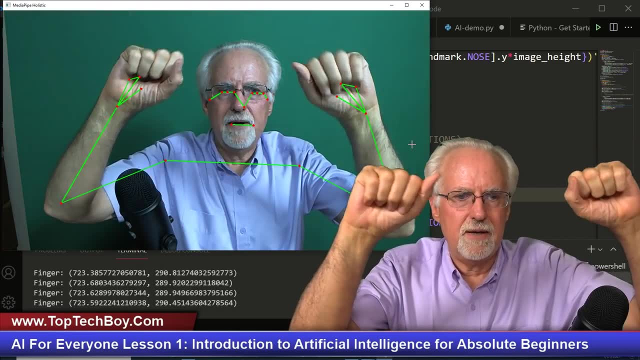 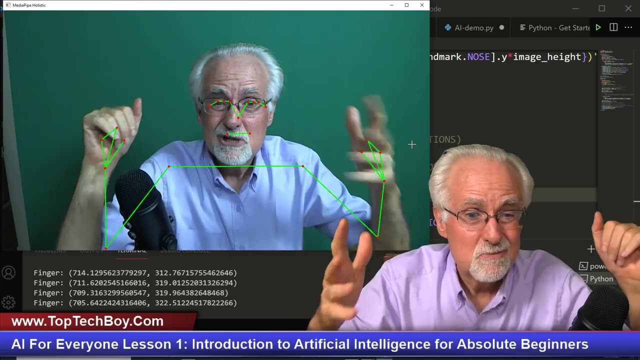 And then I can come in here and give you another quick demo. Okay, And here, rather than analyzing the face, I'm analyzing the whole body. Okay, And if I stood up and dance for you, you know it would show my hips and my knees and my feet, but I will. I'll spare you that, that embarrassment. 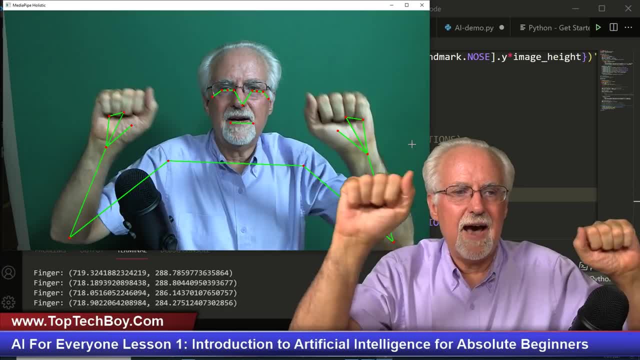 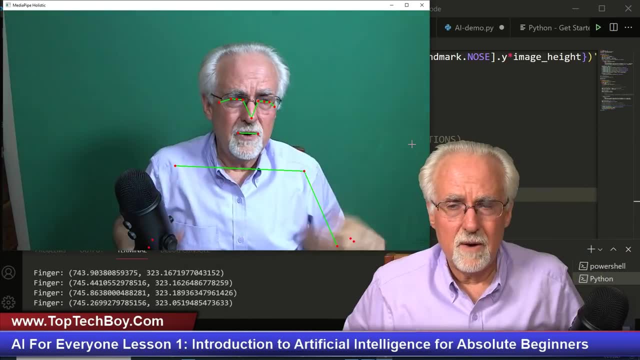 Okay, But you see, I've got the shoulders, I've got kind of the hands. It doesn't have all 10 fingers, but kind of sees the position of the hands, the elbows, the shoulders. If I showed up it would sort of give you all of my major joints. 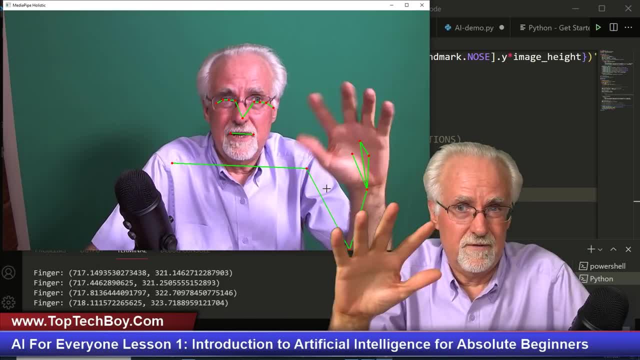 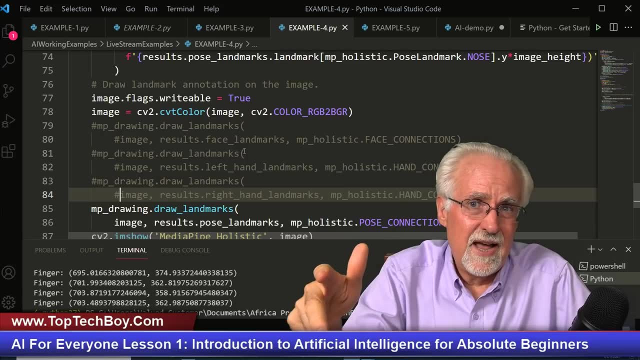 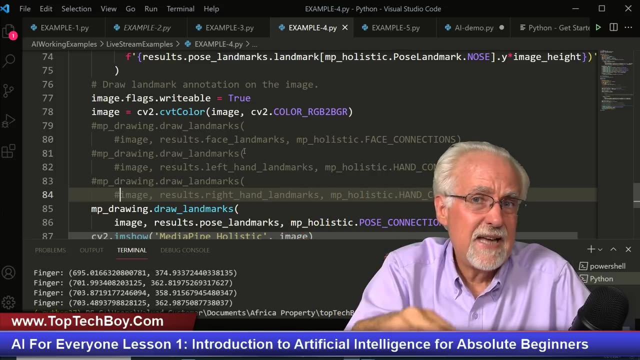 And the amazing thing is I'm getting X, Y coordinates for all of those, So I know where they are, And so that would allow me to write programs that would understand what a person is doing. you know, starting to do things like with gestures, have things happen based on what my hand gestures are or based on what 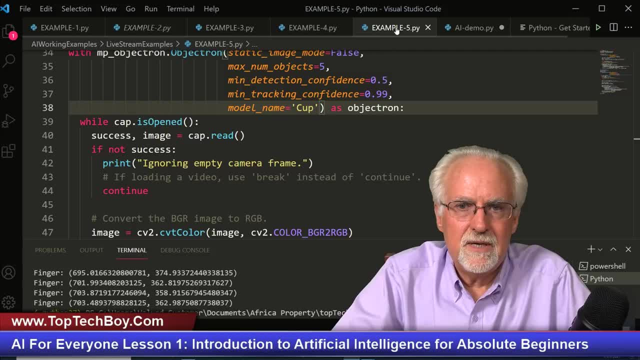 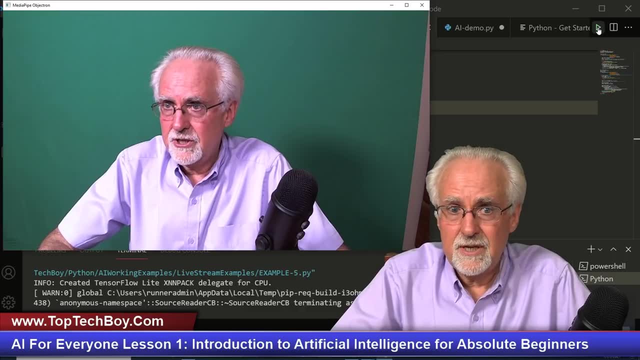 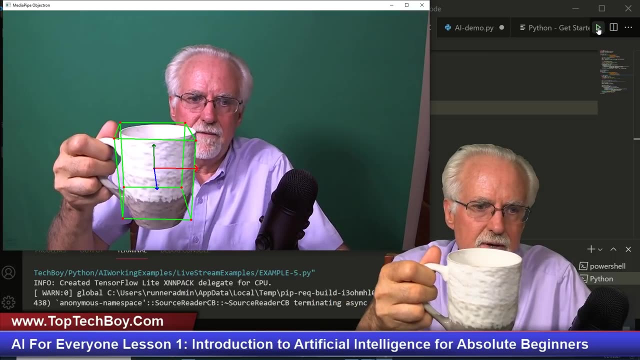 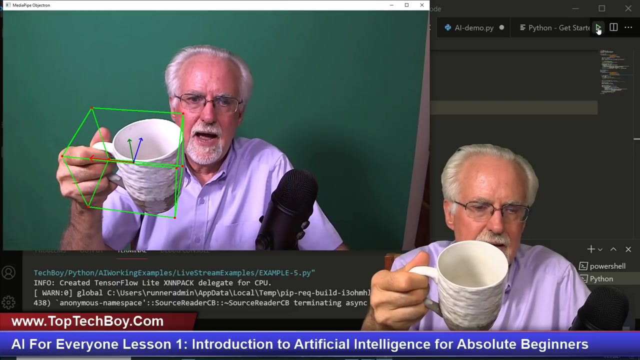 My body motion is start having the Arduino do things based on that. Okay, Let's do one more. here You can analyze not just not just things like uh, not just things like faces and people, but you could look for other things, like a coffee cup, and you can see this coffee cup is a little hard for it to find, but you can see that it is finding and tracking and orienting in three-dimensional space. 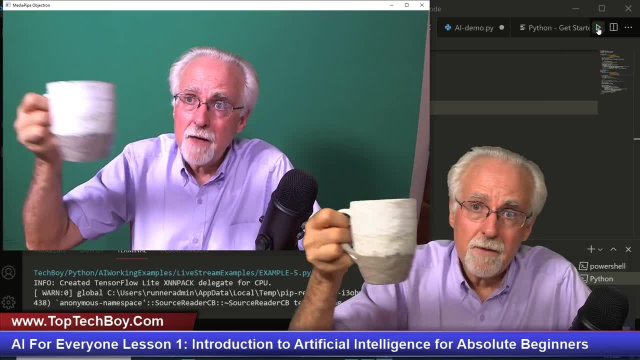 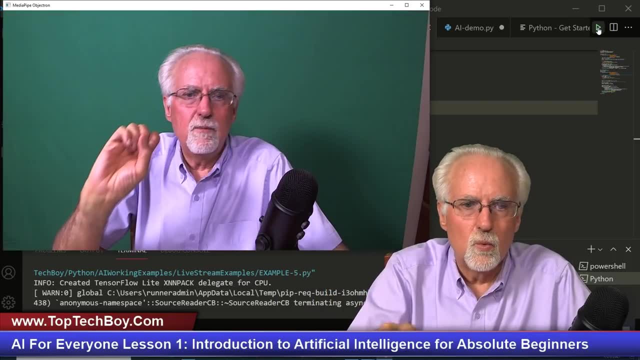 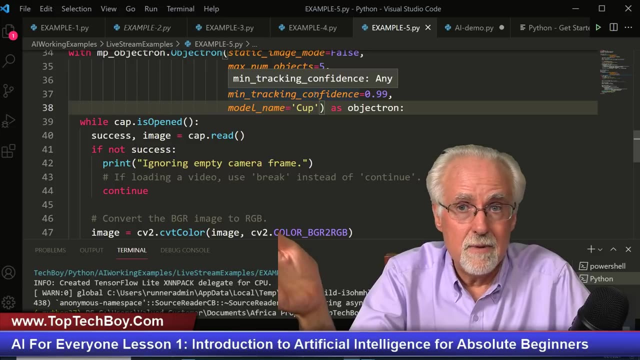 My coffee cup. The coffee cup is a pre-trained model, but we could take that pre-trained model and we could retrain it, and we could retrain it. instead of looking for a coffee cup, we could retrain it to look at a monkey. 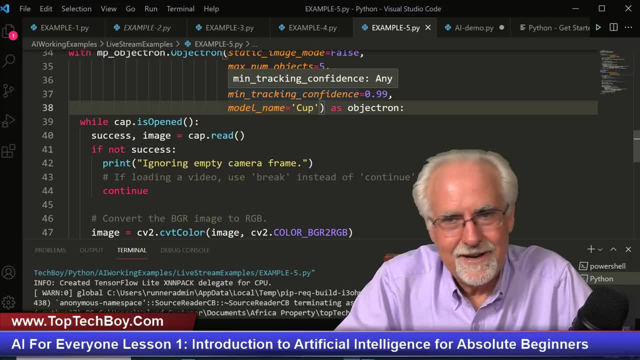 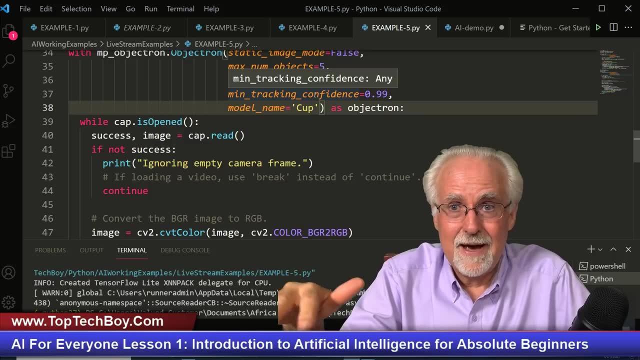 I am having monkey problems these days, though, Yeah. Okay, I know you guys hate it when I digress, but I can't, I can't help it, Okay, So. so I have monkeys that are stealing my food, All right. 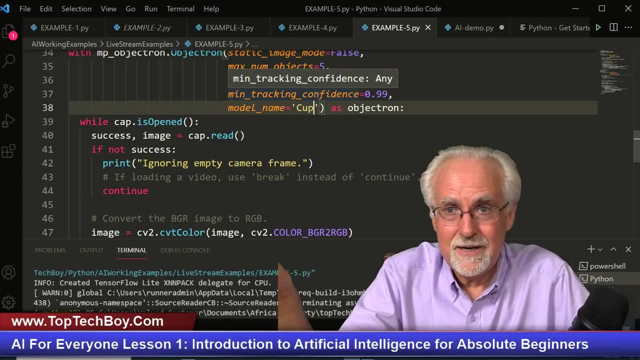 And so I was asking. so I said, ma'am, What happened to this stuff? They said, well, the monkeys, the the the monkeys took the corn. Okay, The monkeys took the corn. and I said, well, how about the dogs? where the dogs, they said the monkeys, were sitting on the porch eating your corn. 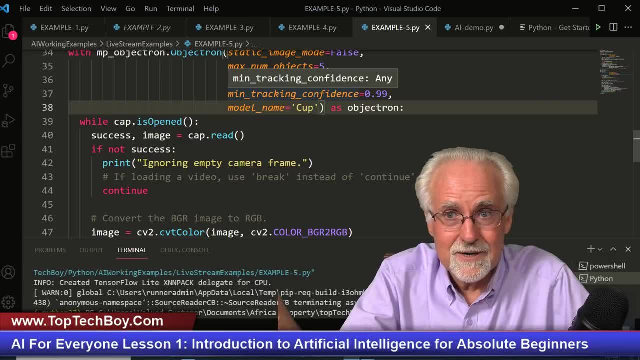 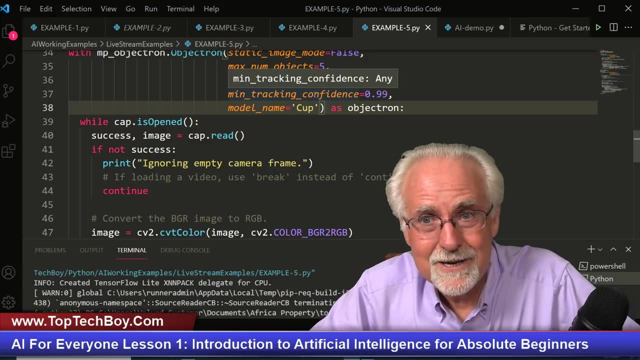 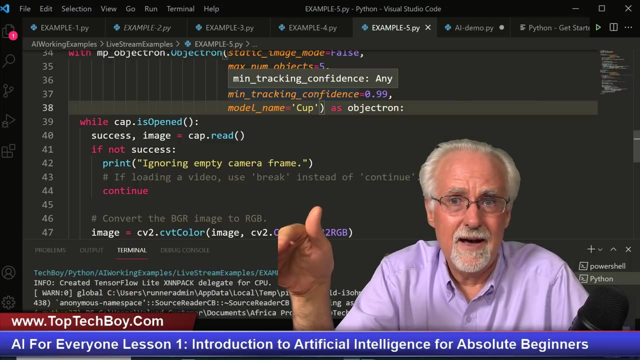 And I said: well, how come the dogs, how come the dogs didn't chase the monkeys off? And what they told me was they said, well, the monkeys were feeding the dogs. Okay, So the dogs have sided with the monkeys because the monkeys are feeding them. but I digress. just, you know, think of the worst pest you've ever had and the 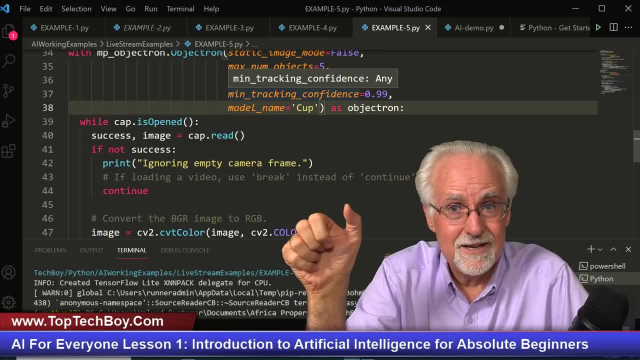 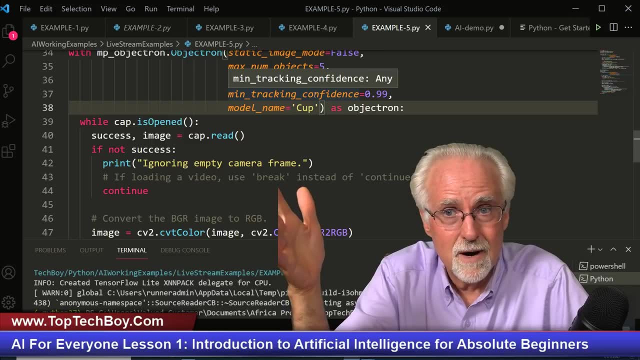 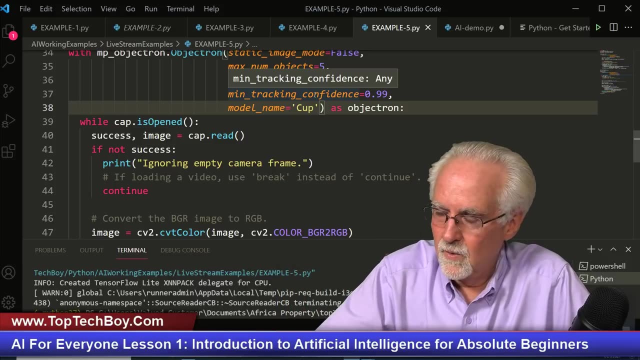 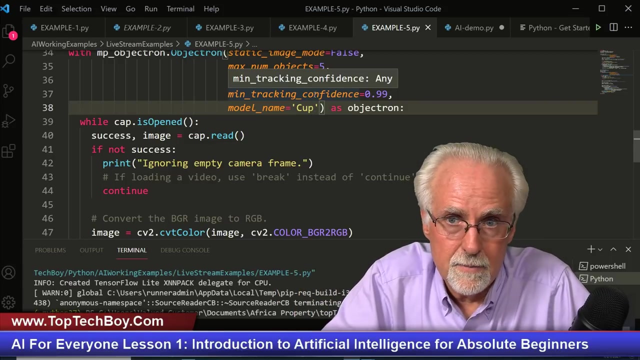 The monkey has a large cerebral cortex and the monkey has thumbs, And so the monkey is really smart and he has thumbs. That means he is a formidable opponent, and I have problems with monkeys eating my food, getting in my garden and stuff. And so I'm thinking about, rather than recognizing a coffee cup, what if I could recognize a monkey and then take countermeasures? just leave it at that? 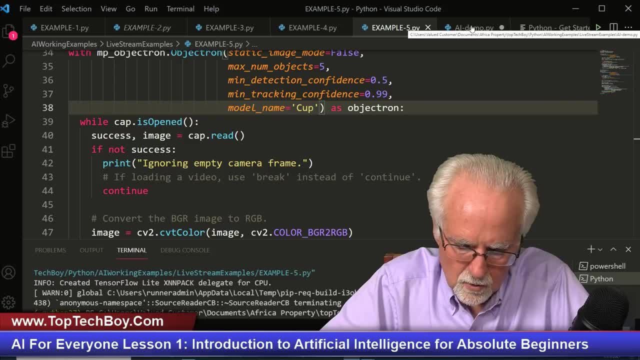 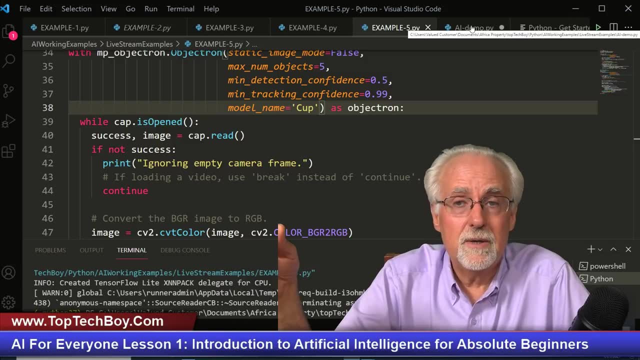 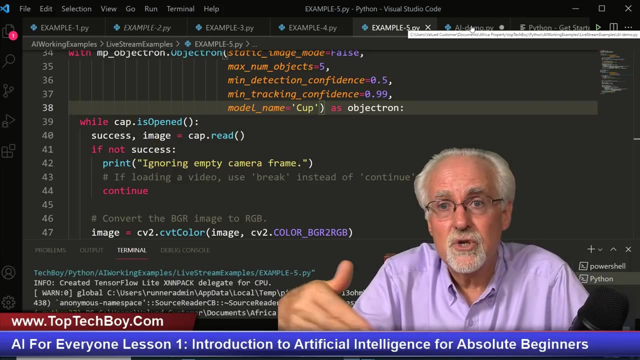 Okay. So, anyway, I apologize that I have digressed like that, but in this, in this, uh, in in these classes, okay, In these classes there are going to be homework, Okay, And so every lesson I'm going to give you a homework, and then usually the next lesson, I'll come back and give you the solution to the homework. 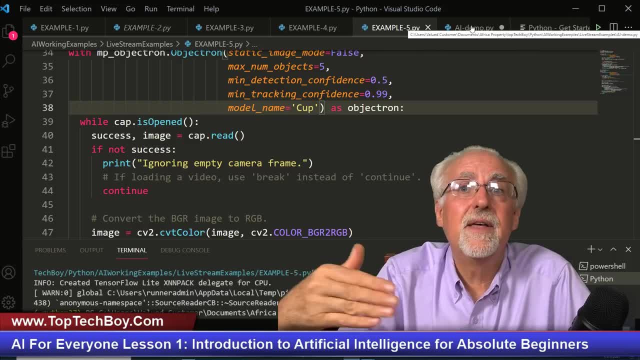 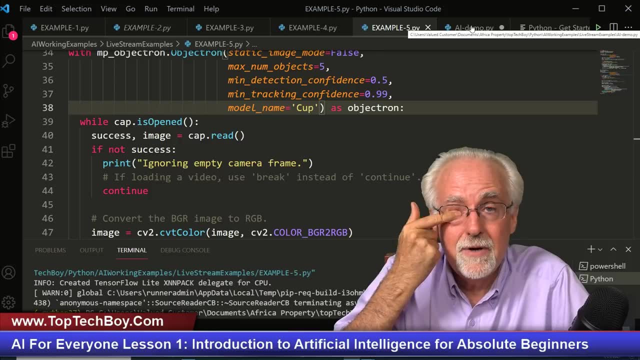 So hopefully you can figure it out. but if you can't figure it out, then in the next lesson I'll do it. But, guys, I need you to really try to do the homework before you just go and copy what I've done, because when you try and when 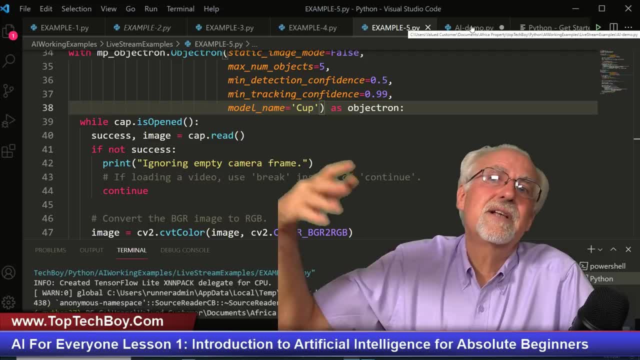 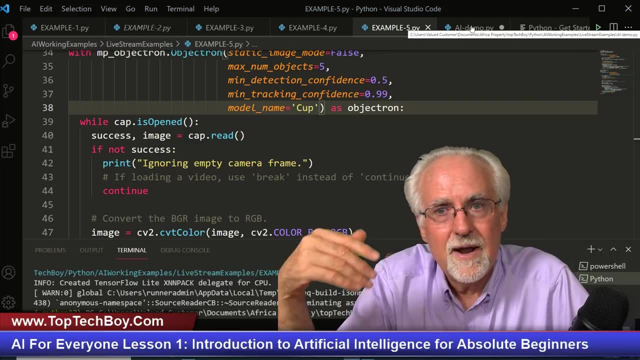 Fail and when you struggle and figure it out, then it's like the greatest joy ever to struggle with a hard problem and then figure it out. Okay, And then, even if you don't figure it out, then when you see me do it, it's like the light bulb will go off. 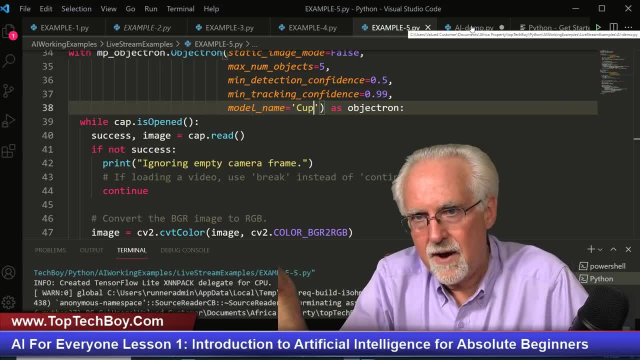 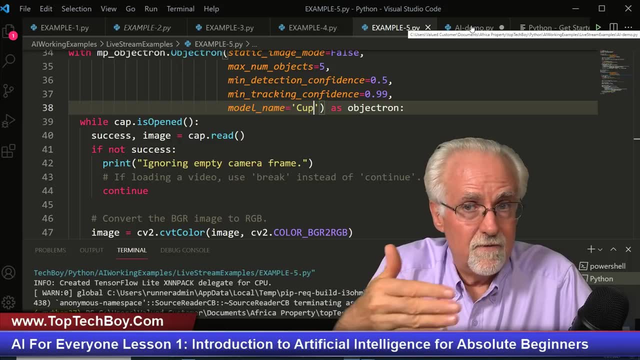 Ah, I see where I was getting stuck and I see how I should have thought about it, And now I see how to do it Now, if you don't do it on your own and you just fold up like a cheap lawn chair and can't do it, 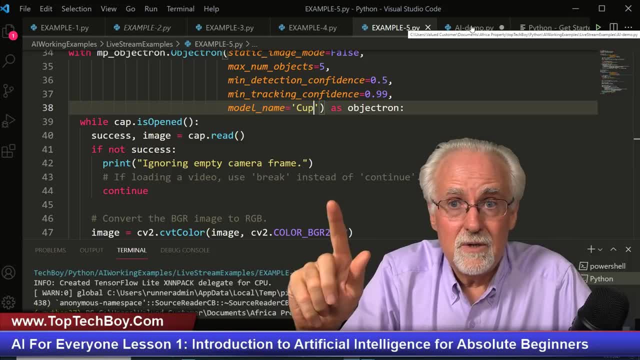 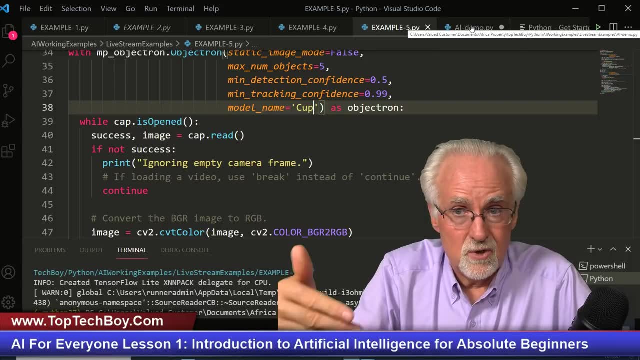 And then, when you see me do it, and then you understand It. what you need to do then is you need to pause the video and then you need to go back and do it on your own without watching me. So you, you, you figured out from watching me how to do it, but you still need to go back and do it on your own without watching me. 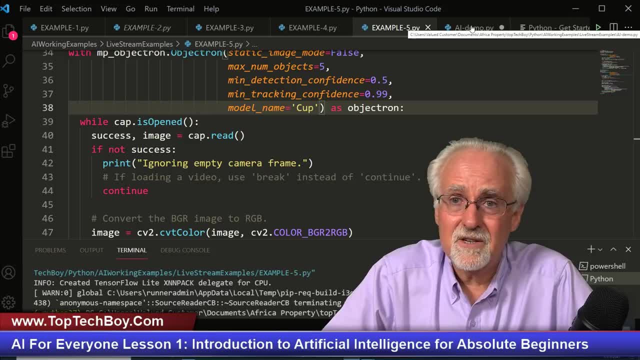 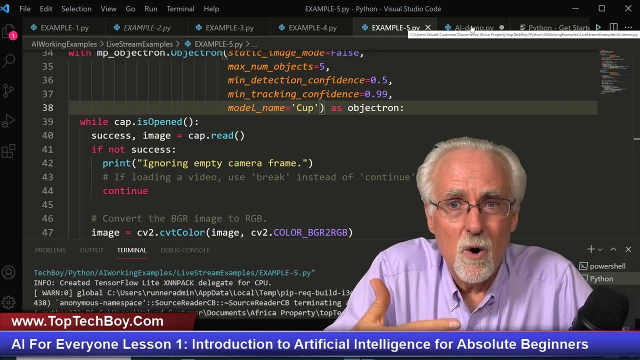 And then you would will have really learned, because the goal of this class is not for you to just copy what I do and impress your friends by copying and pasting what I do, But my goal is for you to go out and be able to do what I can do without me. 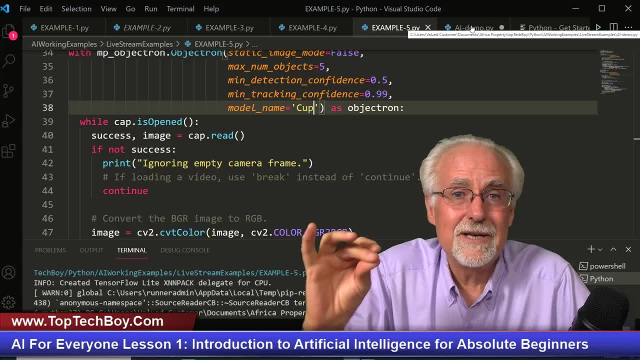 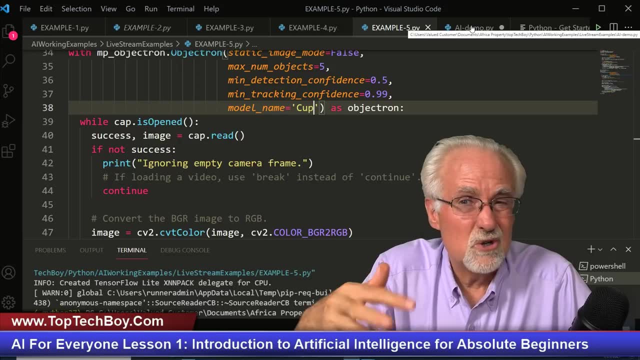 Now I like you following along. You're with me, but I want you to be able to do these things without me, And that's what my goal is. So there will be homework and then the following lesson. I'll show you the solution to the homework. 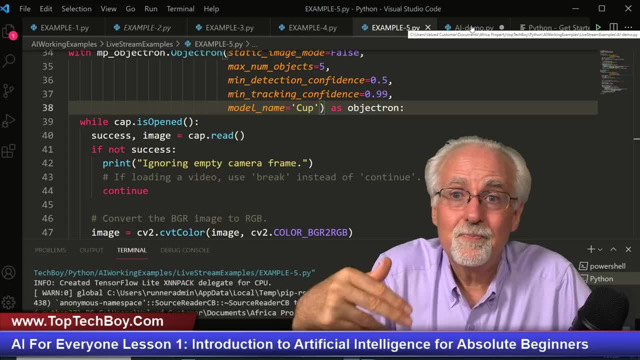 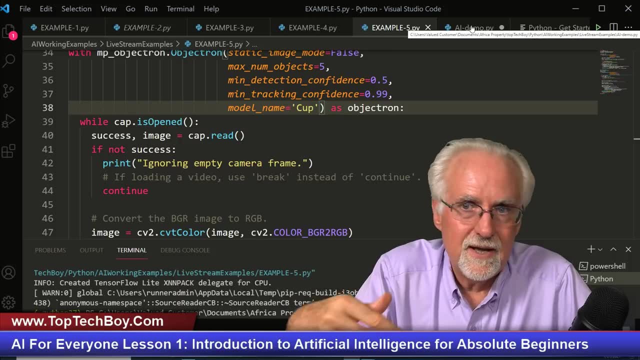 So maybe I'll try to do, if I can. I'll try to do like two lessons a week. in one lesson I'll teach you something and give you homework, And in the next lesson I'll give you the solution. And then the next lesson I'll teach you something and give you an assignment. 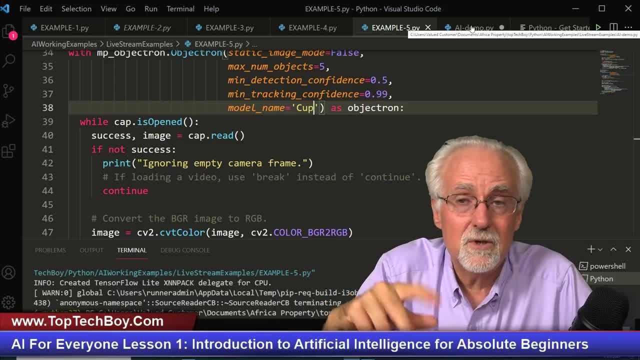 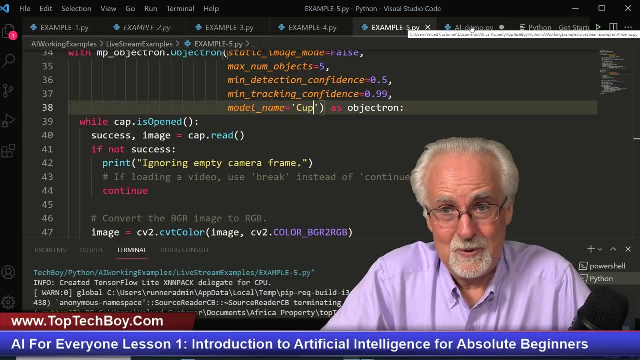 And then the next lesson. I'll give you the solution. Okay, So maybe we'll try to do two, two lessons a week and then always Always learning something new. But since I didn't really teach you too much today, I will, because I am going to give you homework. 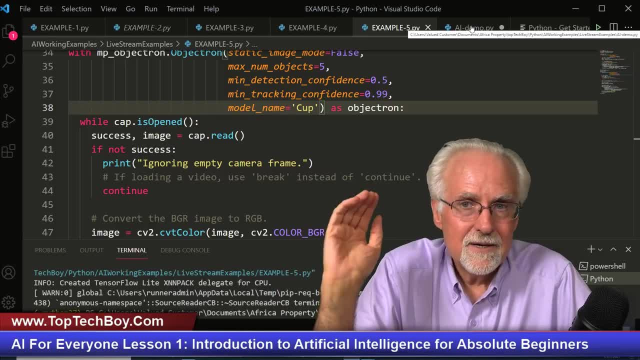 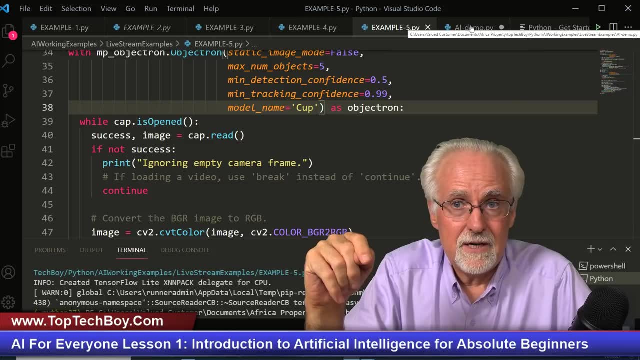 The other thing I'm going to do is I'm really going to try to incorporate math into this, because, darn it, most people hate math, and they hate it for good reason, And the reason people hate math is number one. their math teacher in school probably didn't really understand math. 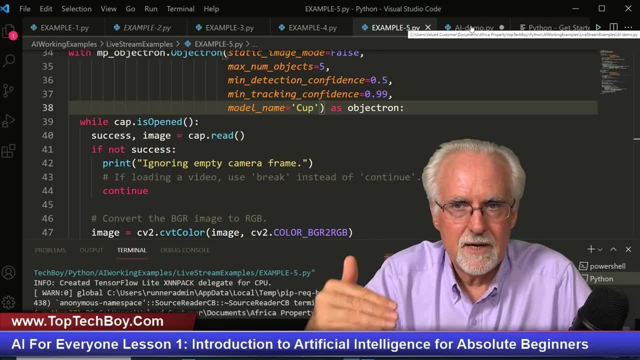 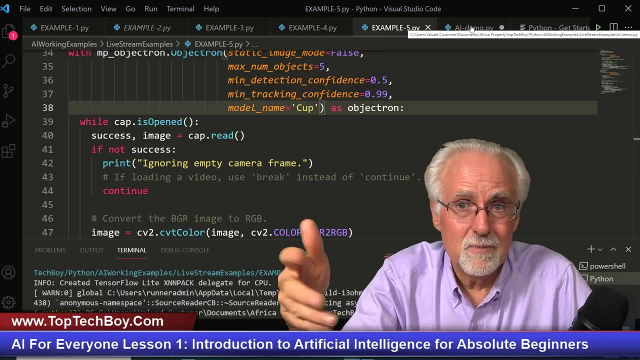 Math teachers are showing you a series of steps and then you're trying to memorize those steps and you're trying to be able to repeat back these steps. You don't understand why the steps are important and you don't understand what the steps mean, but you're just trying to get through math and you hate math. 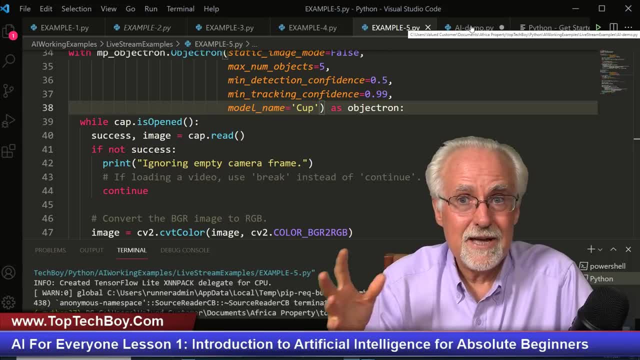 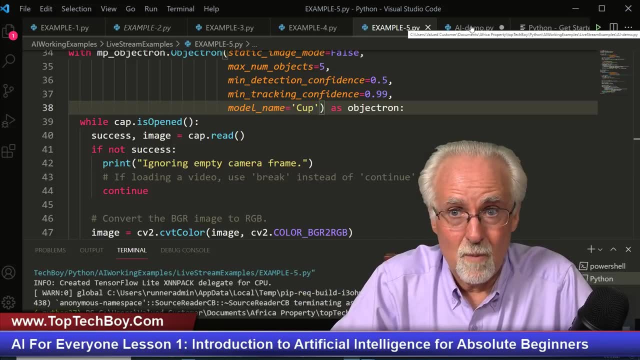 But really the beautiful thing about math is there's problems and you can't. there's important problems, important things you want to do in a project and you can't really do them unless you understand the math. So I'm really going to be trying to incorporate math and physics into this as well in a fun way. 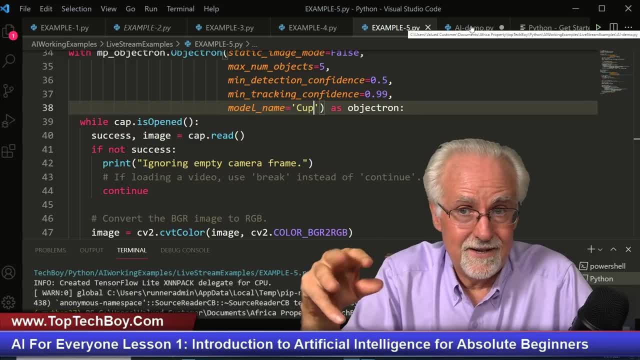 Okay, So that some of these things are going to require you to, to, to kind of know some math, And then I'll also be teaching you that math. So we're going to be doing a little bit of that, Okay, A little artificial intelligence. 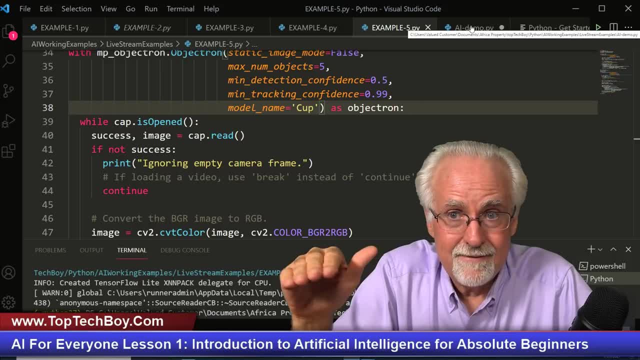 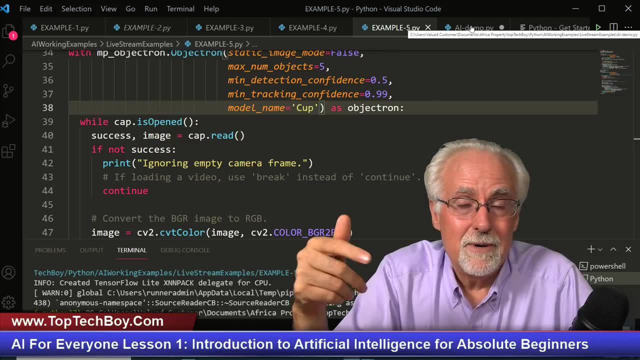 We're going to be doing a little physics, We're going to be doing a little math, but we're going to be having fun as we do it. Okay, And so that's kind of what you can expect in this class: whole lot of fun, but you're going to be learning some important stuff, but you really need to be trying to do the homework that I give you. 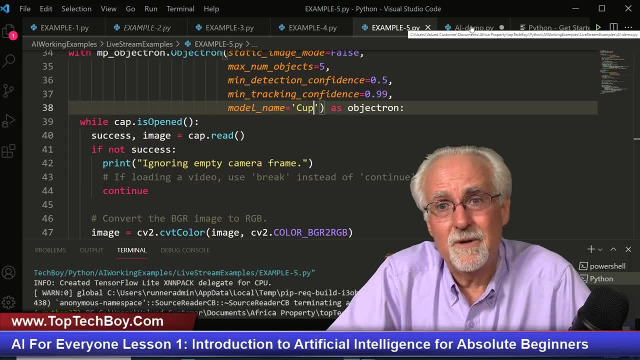 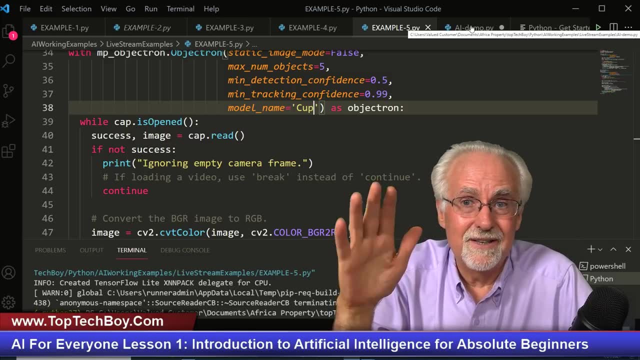 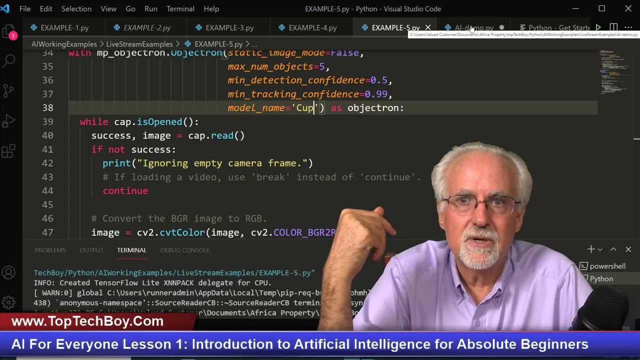 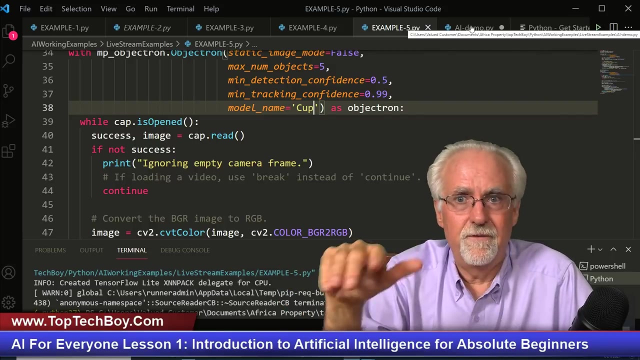 But for today, what the homework assignment for today is. I've told you a little bit about artificial intelligence. Well, I need you to write a paragraph in the comments down below, or at least a bulleted list, but maybe a paragraph Where you've actually thought about this: what do you think are the three biggest potential benefits to mankind that artificial intelligence might have, like ways that you could use it to that could fundamentally improve mankind? 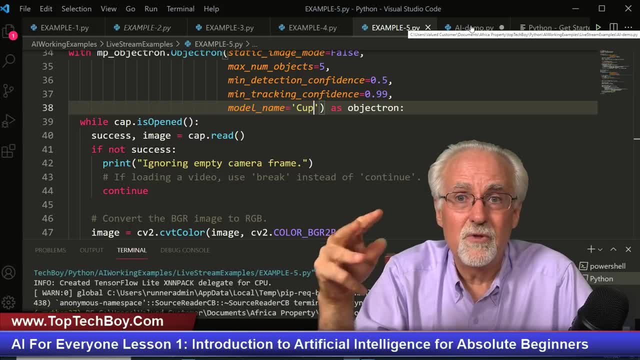 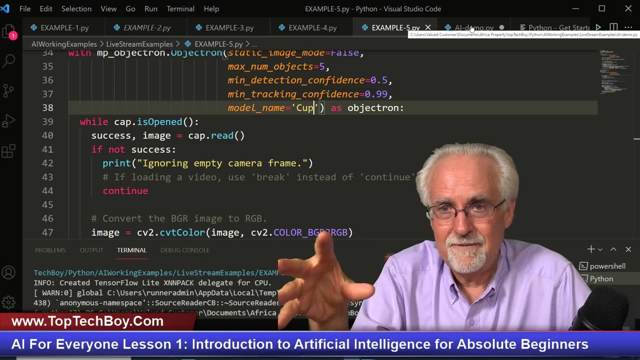 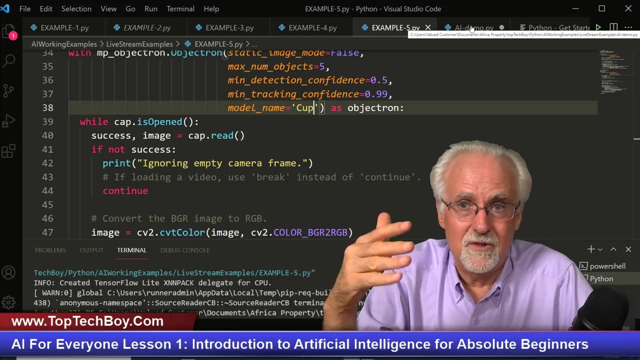 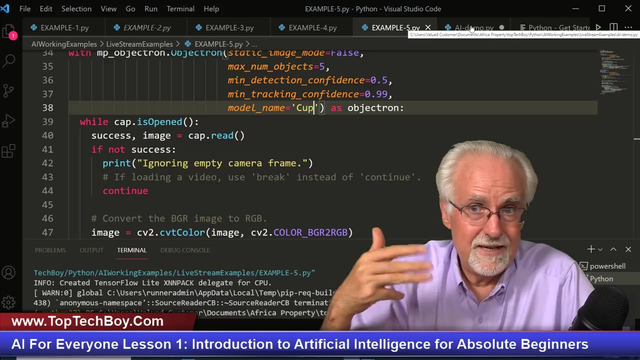 And then the second thing I want you to do is tell me what you think the three biggest risk or the three biggest threats of artificial intelligence are. Okay, The three biggest advantages of artificial intelligence, how it could impact positively mankind, The three biggest risks- the way that it could threaten mankind- and then leave a paragraph down below, or at least a bulleted list of the three- uh, you know good things- the three threats that artificial intelligence have. 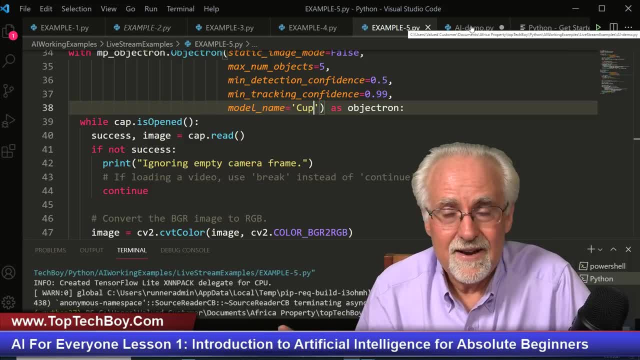 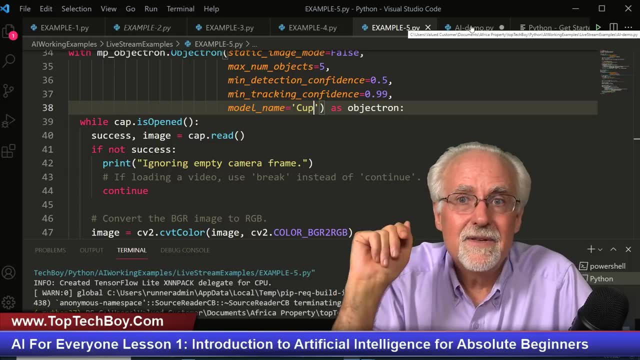 And then the conclusion about overall: do you think that net net, it's worth it or net net, We should just hope it goes away and run from it. So let's get your perspective. And then the second assignment is: read the other comments down below and respond.